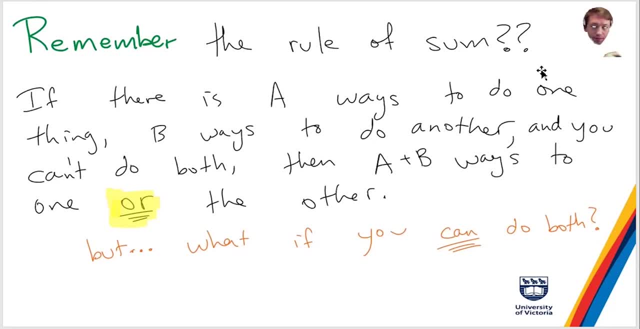 So remember what the rule of sum said. So what it said is that if there's A ways to do one thing, I like this example somebody gave in the class- the first class of this year, this term- which is like: if there's A ways to stand up, there's B ways to sit down. it's impossible to stand up and sit. 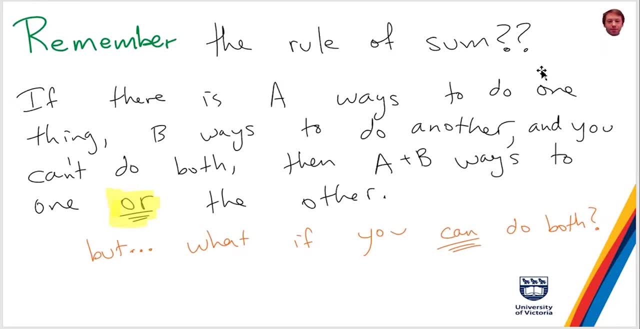 down at the same time. So the number of ways to either stand up or sit down is A plus B. right, But in general if there's A ways to do one thing, B ways to do another, you can't do both. 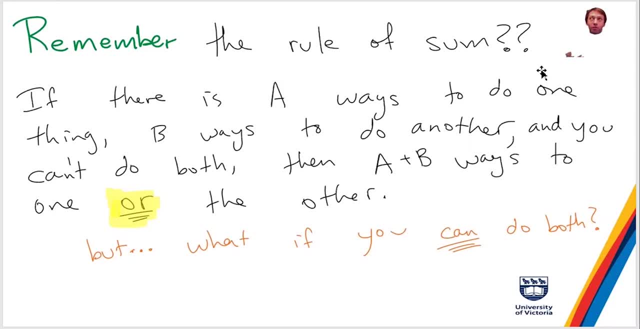 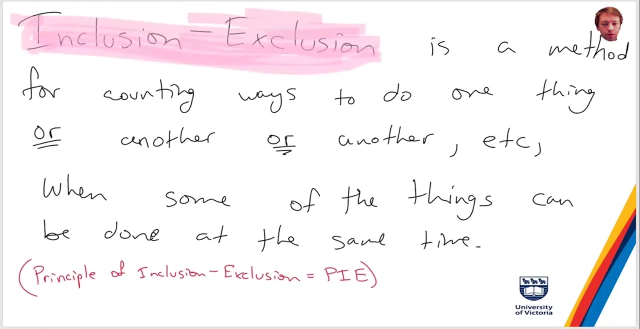 then there's A plus B ways to do one or the other. But now the question becomes: what if it is possible to do both? So then now, how many ways are there to do one or the other? Okay, so that's the kind of question we're going to address today. So the inclusion-exclusion. 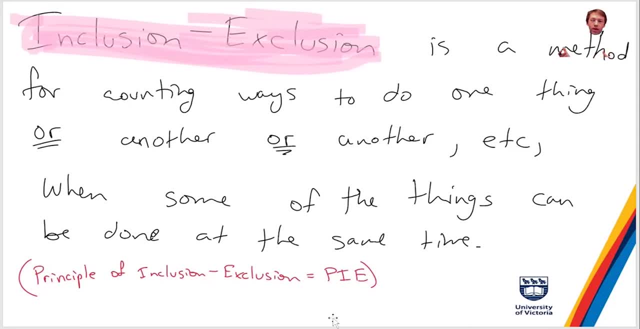 principle. So this gives you a method for counting ways to do one thing or the other, or maybe multiple different things, right? The number of ways to do A or B or C, and so on. Yeah, right, So, and the key thing is that we want to count this, even when some of those 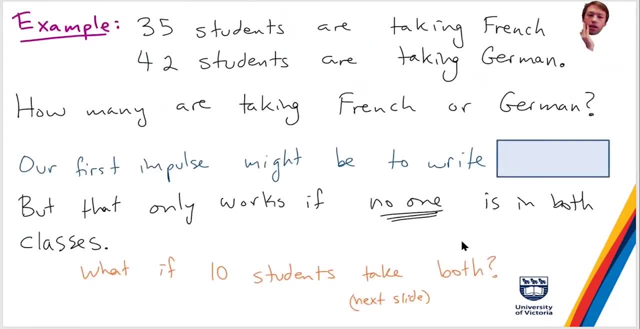 things can be done at the same time. Okay, so here's an example to think about. So suppose that there's 35 students taking French and there's 42 students taking German. Figure out how many students are taking French or German right, And we don't want to count a. 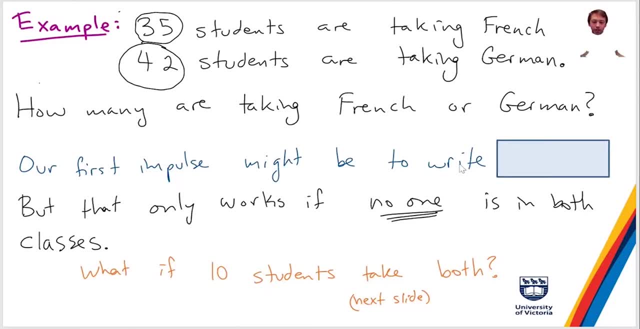 student twice. So we want to say how many yeah, in total. if I put all the people who are taking either French or German, I put them all into the same room. how many people are there? And, like the first impulse, like you feel like you want to write 35 plus 42, right, You would think if 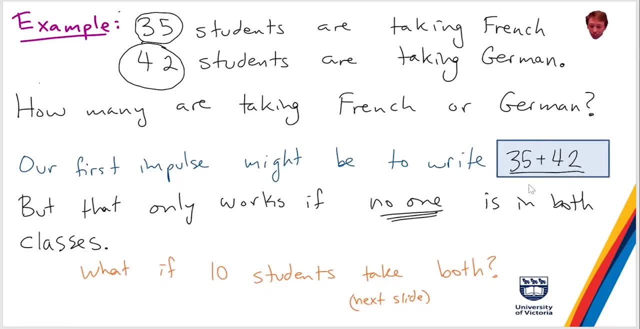 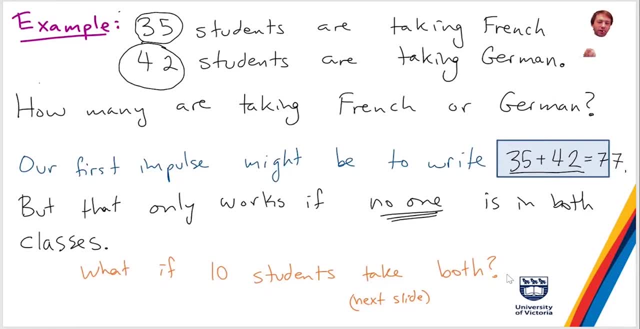 know, which is 77, right, But that's not quite right, Because what if one person? you know, what if somebody is in both classes? Right, Because you're not gonna. if I take all the French and German students and put them in a room, that person is not going to appear twice, So you have. 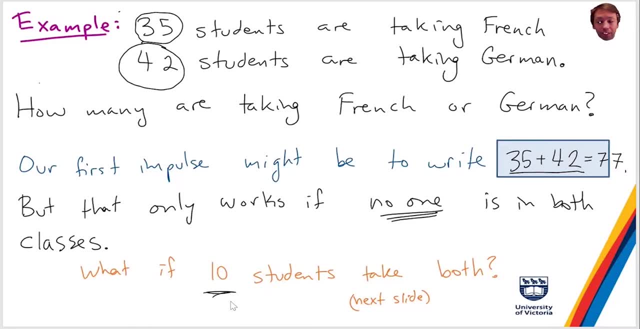 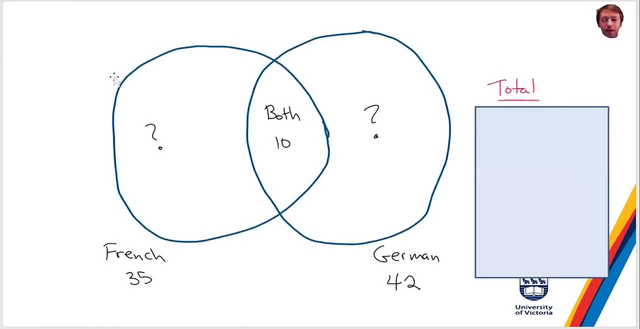 to be a bit careful. So, for example, if there are 10 students taking both, we have to think a little bit. So here's the kind of way of thinking of it. So in total, so imagine: yeah, so this is this circle here. So it's the way to think of it is in terms of a sort of Venn. 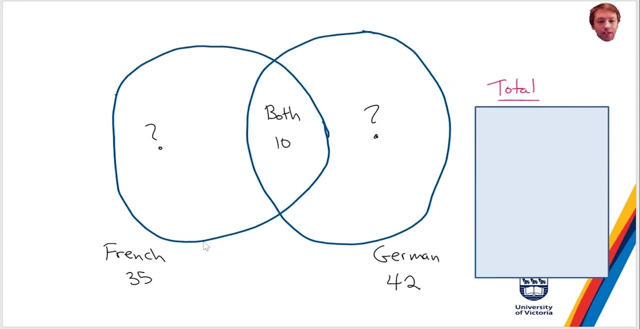 diagram, right? So this suppose this circle here, maybe I'll highlight it- Suppose that this circle contains all the French students, students taking French, And suppose that this circle contains all the students taking German. And we know that there are. ooh, it's interesting When I overlap the. 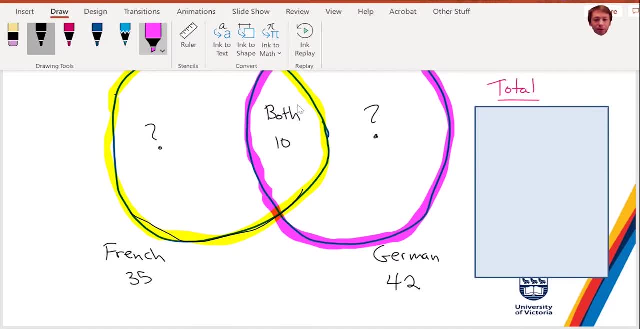 highlighters. it combines the colors And suppose we know that there's 10 taking both. So how many students are there in total? So can anyone tell me? I don't know, I don't know, I don't know. Does anyone have a guess at the answer? Yeah, that looks right. So there's various ways I could. 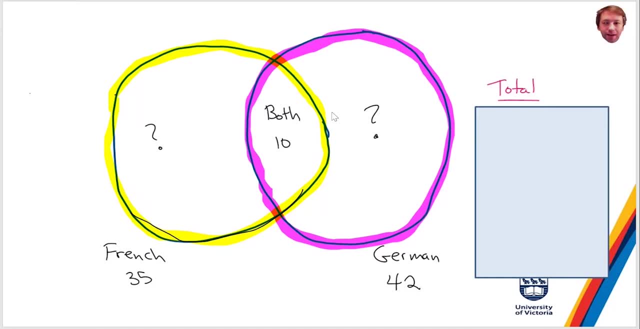 try to work this out. Let's, let's. so I'll do it one way and then- but this is not the way I would suggest, But then I'll think about it another way. So I mean one way to do it is. 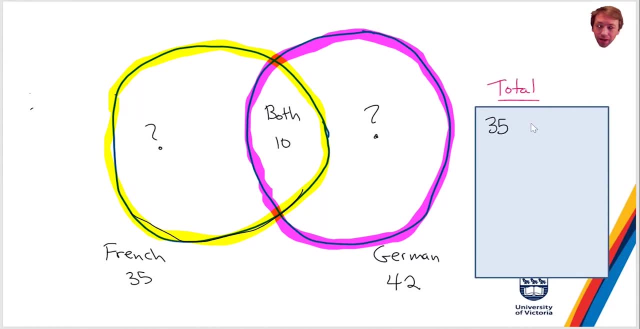 you could say: let's say you know there's 35 students taking French, right? So we've counted each of those ones once. And then we want to count all the ones taking German, but we don't want to recount these ones, right? So you could then go and say like 42 minus 10. 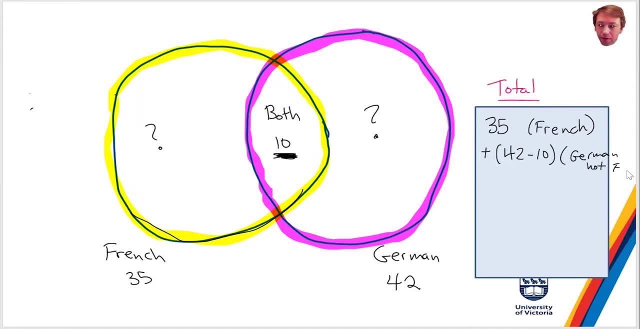 taking German and not taking French. So these are like new students, the ones that you haven't counted yet, And yeah, that'll be 67.. In general, though, what you can do, so, rather than thinking through this step by step like this: yeah, what we're going to prove, is that actually what you? 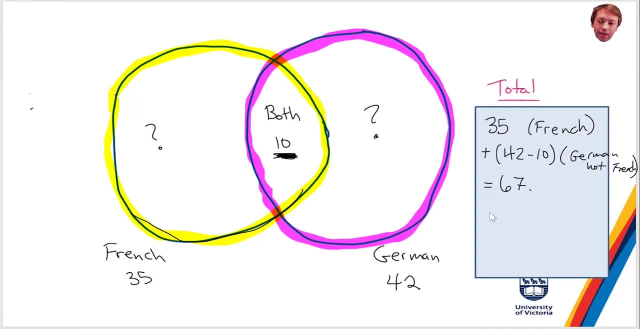 can do is you know there's, there's a simple formula that it's you know you can do this. you know the number of things in the first set plus the number of things in the second set. So this is always going to be the case. So 35 plus 42, and then you subtract the things that are in. 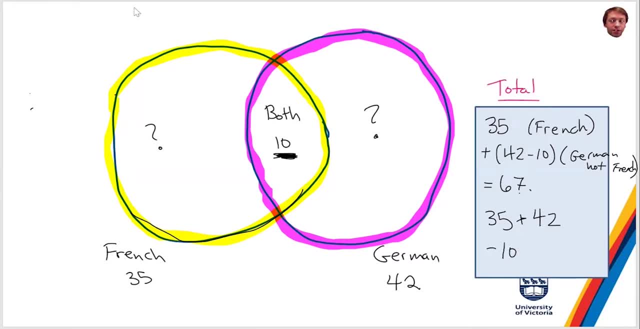 both. So. so this is the kind of answer to like what if you have something involved, something similar to like the rule of sum, where you you're taking, you're trying to count A or B, but A and B can happen at the same time. What you do is you add up, yeah, the number of the first type of 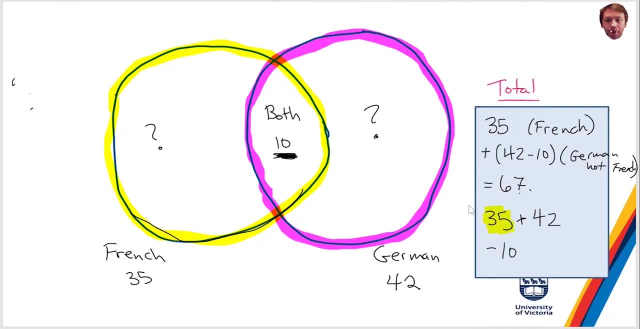 things you want to count, Plus the number of the second type, minus the number of things which are both both types at the same time. Is this example clear? Okay, Thanks for the participation giving the answer in the chat. But yeah, so we want to kind of think about this, not only for two sets but in more generality. 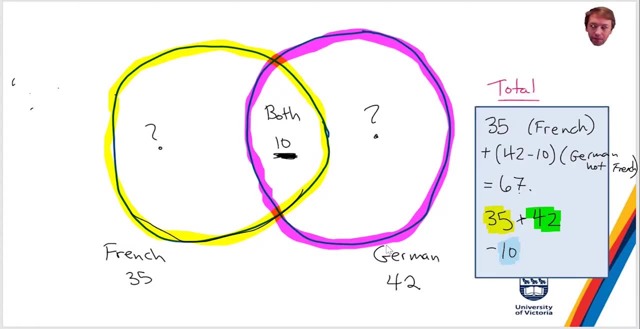 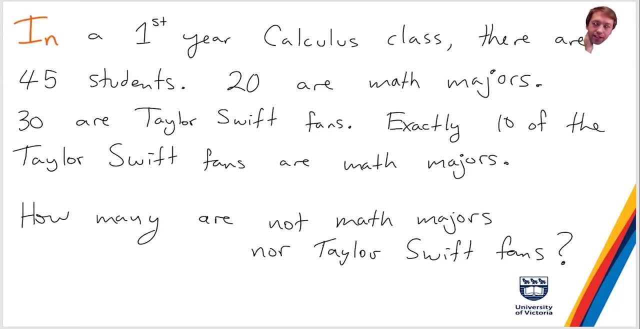 So I'm going to try to build up the kind of concepts. Yeah, So another example. So in a first year calculus class there are 45 students, 20 of them are math majors. So 20 math majors, 30 of them are Taylor Swift fans, It's quite a large proportion of the class, Exactly. 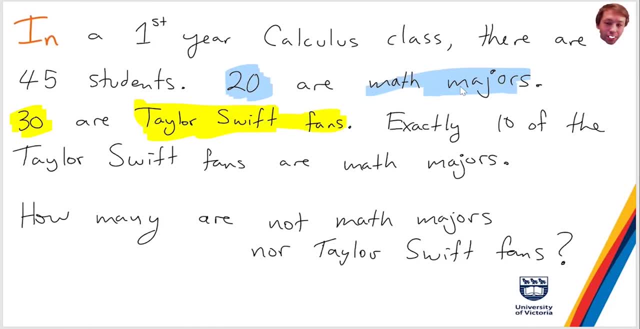 10 of the Taylor Swift fans are math majors. Okay, So yeah, 10 of them are both, you know, Taylor Swift fans and math majors. How many of them are not math majors, nor are they Taylor Swift fans? So how many, yeah, How many are neither? And yeah, 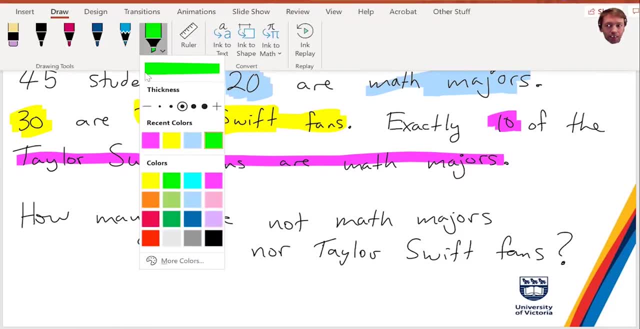 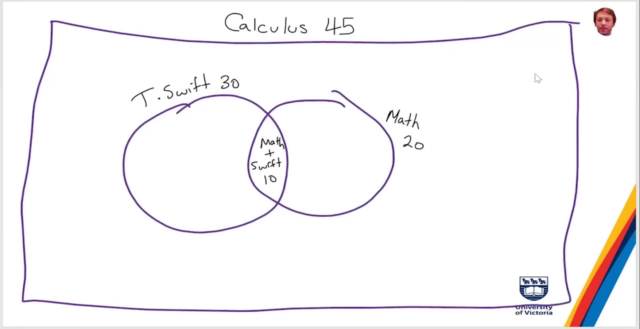 it's important here. There's 45 total students, Can anyone? so, given what we've learned, might be five. Let me let me think through the calculation. Yeah, So actually, do I have this in the next slide? Okay, Yeah, So, yeah. So this is this calculation in the in the chat looks correct, So so right. 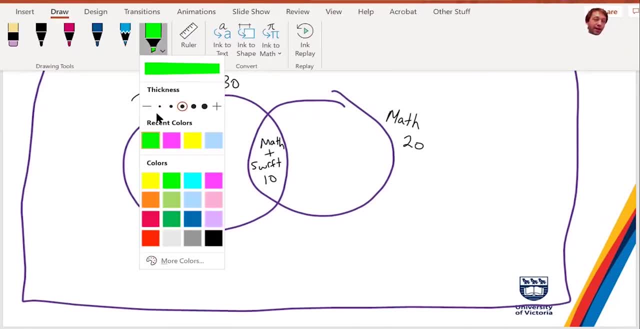 So what we want to do, we want to count the people who are not Taylor Swift fans and not math majors. but what we should do is count the compliment right, Because yeah, So if we count, let's say we count the ones that are Taylor Swift fans. that's 30. We've got the ones that are math. 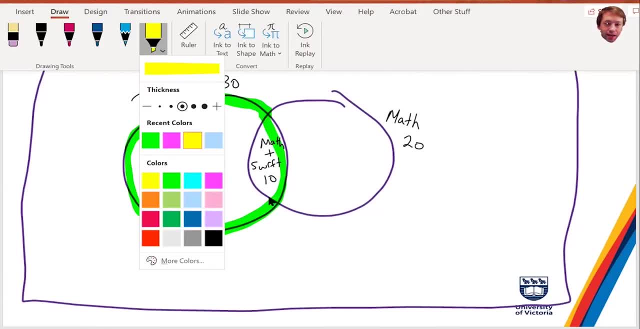 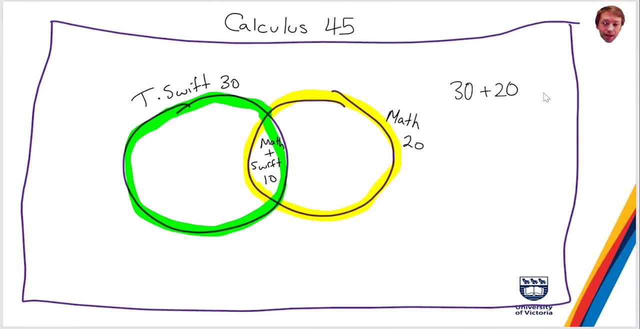 majors, that's 20.. And then you've got the intersection, which has size 10, right? And so by the formula we kind of derived before we've got, 30 plus 20 minus 10 is 40 are either math majors, or I think they call them Swifties, right, Taylor Swift fans. And then 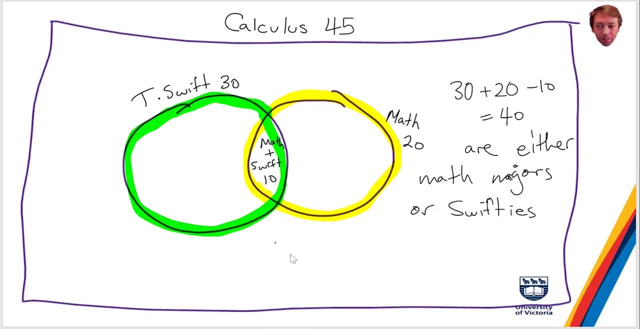 yeah, we want to count the ones that aren't that. So we just subtract, right, So 45,. there should be more in a calculus class. You would think that there'd be more math majors than Taylor Swift fans. but Hey, this is a, this is yeah. everything doesn't go as the way you. 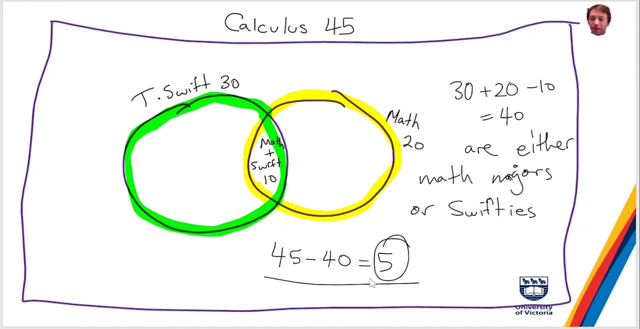 expect. So anyway, so the answer is five because, yeah, when you count up all, the all of these things that are one or the other and you need to subtract the ones that, yeah, you need to subtract that from the total to get the ones that are neither. Okay, cool. 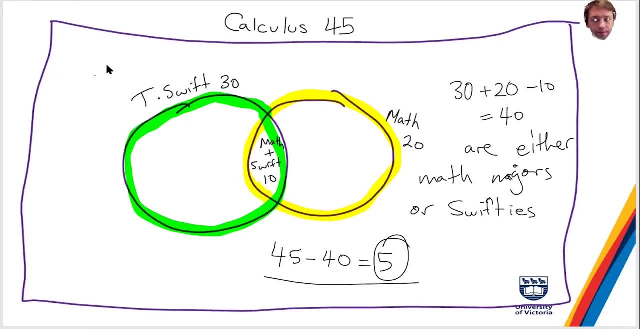 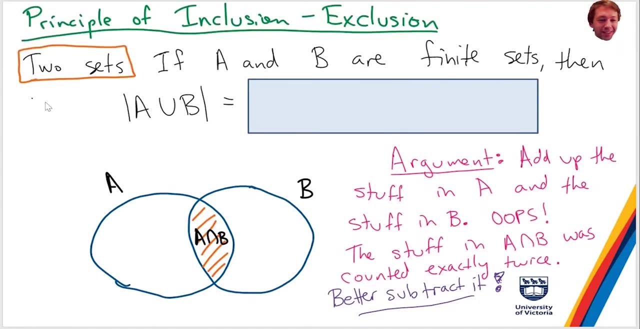 Any questions about any of this? Okay, Math is greater than Taylor Swift. Well, yeah, I don't think the world would agree, though I think this is a a kind of biased sample- the people who are in a math class- But yeah, I think, if you ask a person on the street, 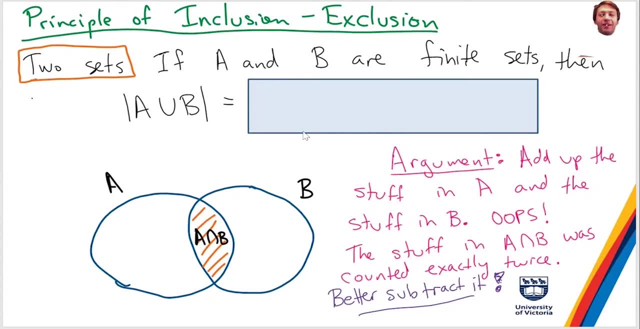 they'll say that math is way worse than Taylor Swift. Okay, So yeah. so just the general principle that we're dealing with here in kind of mathematical notation, is that if A and B are finite sets, so for example, A could be the math majors, B is the Taylor Swift fans or A is the French students. 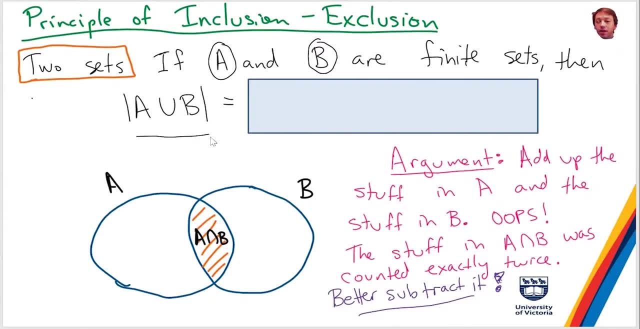 B is the German students. then the size of the union of A and B. the union is, of course, the set of things which are either A or B. B is the size of A plus the size of B minus the size of A intersect B. Is everyone okay with this? 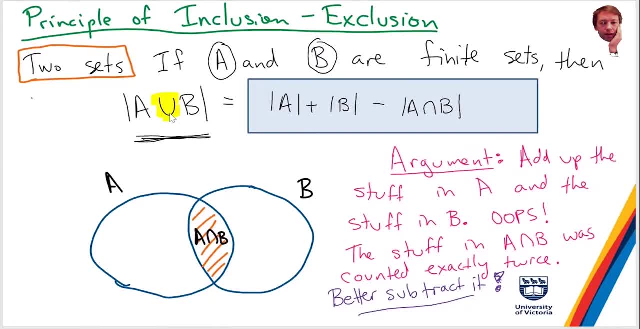 notation union and intersection. Okay, good, So hopefully this is clear that this is what we've been doing right? If I take French or German, you know class, it would be the number of French people in the French class plus German class, minus both. Now what's an argument for? 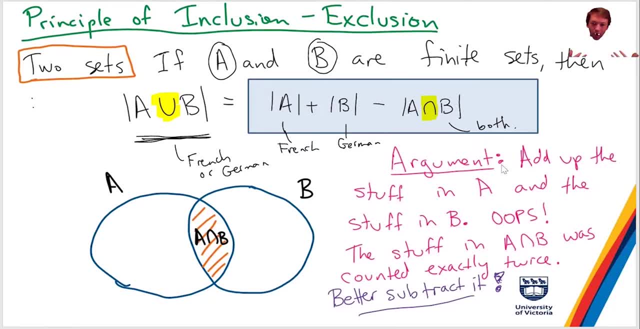 this. Well, I think it's a good argument to like explain why this is true in general, Like why, you know, I've we've kind of done some examples and it looks like this is true. you know, from the. 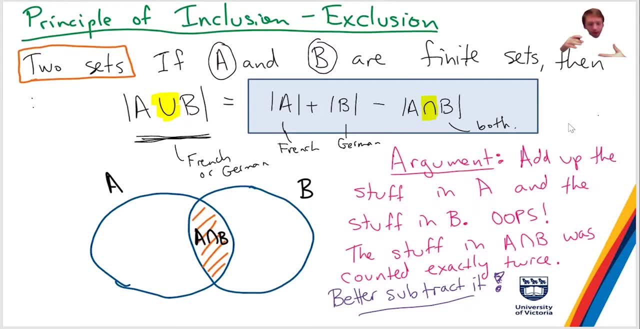 examples. but let's just kind of explain why this is true, right? So? so imagine, you add up all the stuff in A, so add up everything in A, I count everything once, and then I count everything in B once. So that's what we're doing, by taking the size of A plus the size of B. you know, right? So this 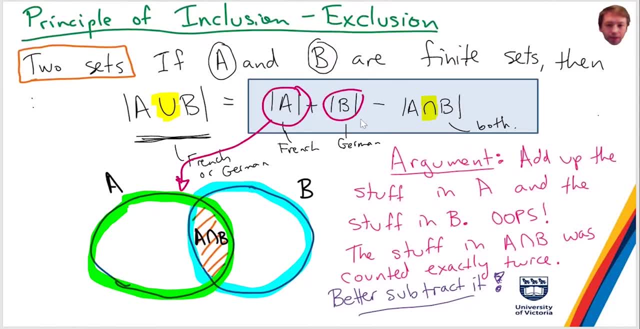 this quantity, the size of A, counts everything in A once. this thing counts everything in B once. But then we look at the intersection and we can just tell like how many, if I have somebody in here, how many times was it counted? Well, it was counted exactly twice, right, It was counted once. 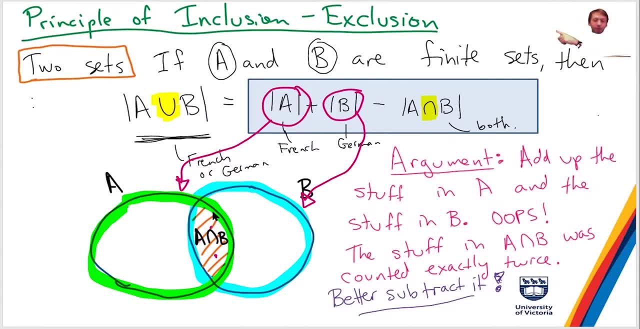 from the perspective of A and once from the perspective of B. Okay, I don't know what I'm doing with my hands here, But, yeah, Right, So. so that's like. so, basically, if I count up A and B. 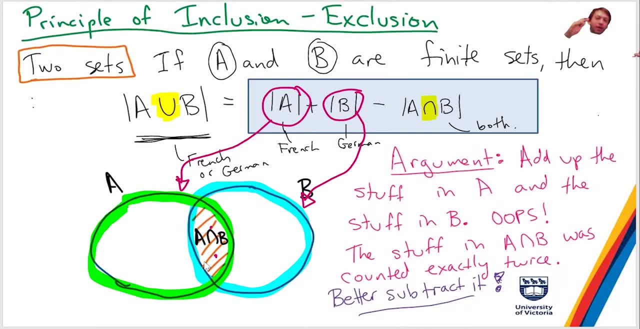 like I've got pretty much the right answer, except what I've overcounted is everybody in the intersection got counted twice, But so to fix it, all I have to do is subtract that amount. So so yeah, that's what I'm trying to explain here. So the stuff in A intersect B was counted. 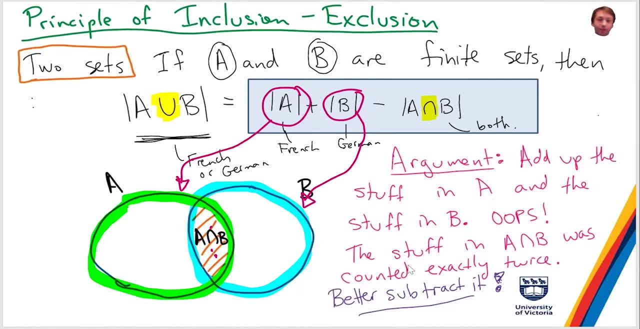 twice, so we better subtract it. And then, once you subtract it, then all that stuff was counted once, and now everything was counted once and we're happy. Is that clear? Okay, so that's the most basic case is when you have two sets, But we want to kind of understand this- when you have lots of different. 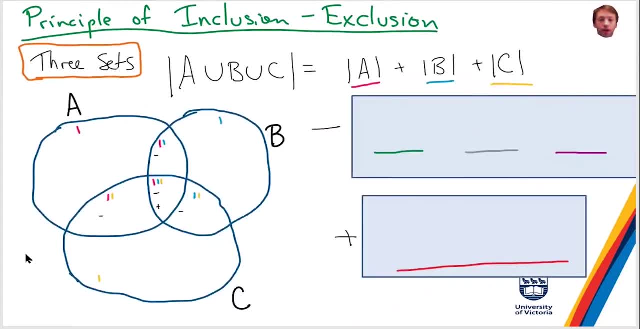 sets which might interact in complicated ways. So let's take one step in that direction. Just think about three sets, Okay, so here's what. let me try to. kind of not sure if this is going to help, if this picture is clear or not, But let's, let's try to think through what the answer is here. So 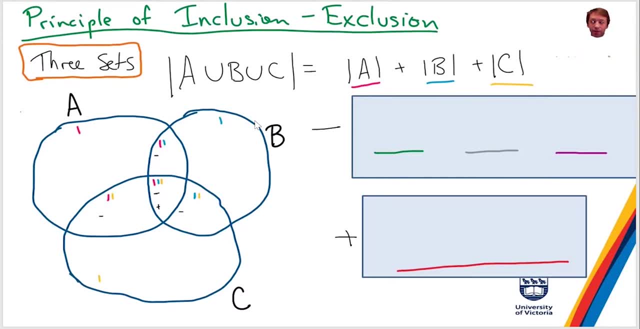 I'm. I've got three different sets. For example, if we want to think about the classes right, A could be the students in French class, B are the students in German class and C are the students in Japanese class right, And we want to say how many are in at least one? how many students if we put them all? 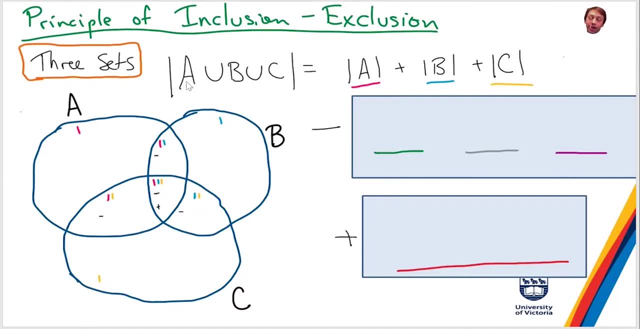 in a room, like all the French, German and Japanese, like language students. we put them all in a room, then how many students would we have? Okay, so, and the way to count this. so what I'm going to do is I'm going to say, okay, how many French students are there? It's the size. 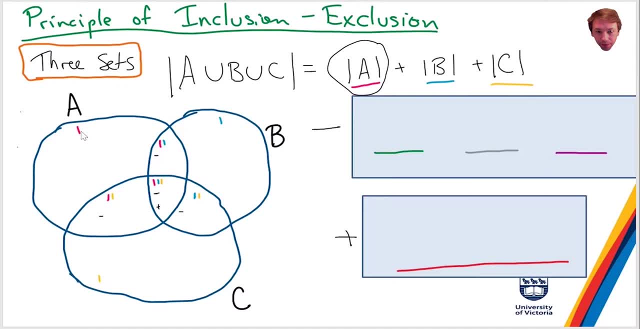 of A, And so I've underlined this in pink And so, basically, I'm in this picture, what I'm saying is in the pink. like by counting this, the set A, I've counted each student in these groups once. 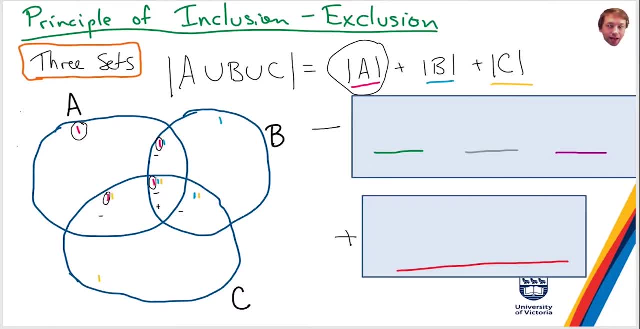 or each, yeah, each thing, each thing in A. so A is all of this stuff, everything in there got counted once. Is it clear what this picture is trying to say? Like, like, for example. this is the set. like this thing in the middle is A intersect B. 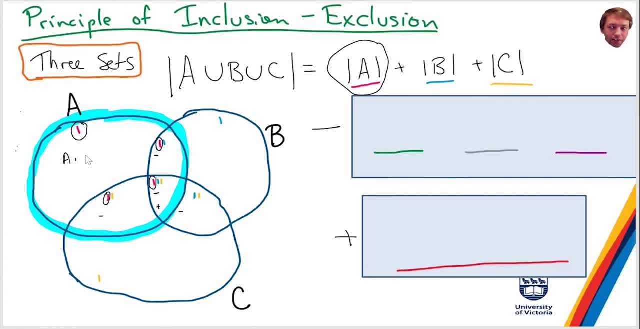 intersect C. you know, this is the stuff in A, not B, not C and whatever. Okay, And then when I count B, I'm going to get everything in here once. everything in here once. everything in here gets counted once. and here gets counted once, right. And then C is similar. everything in 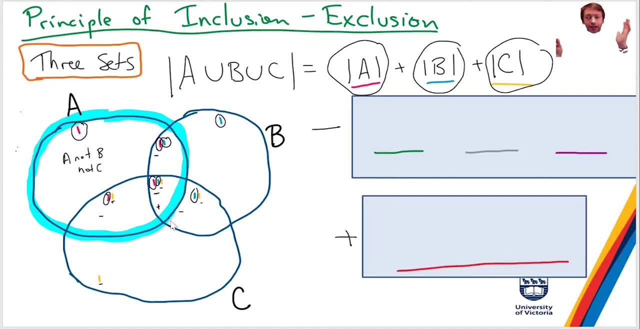 you know these places get counted once, So I can see that everything in like these, like this set here, and this one here and this one here, everything there is fine, I've only counted it once, But then you can see that all of like these little segments, I've counted everything. 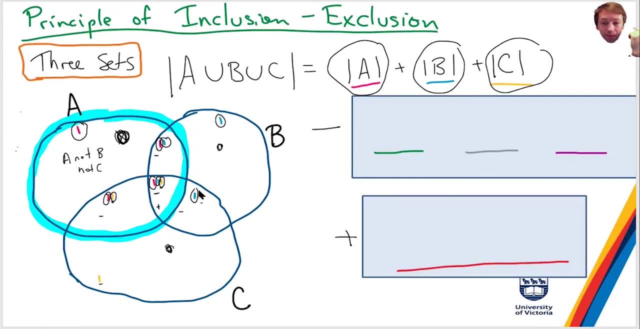 too many times. In fact, here I've counted everything three times as much as I should have, And here I've counted everything twice as much as I should have, and so on. So so what I'm going to do next is I'm going to subtract A, intersect B, And it might not be clear. 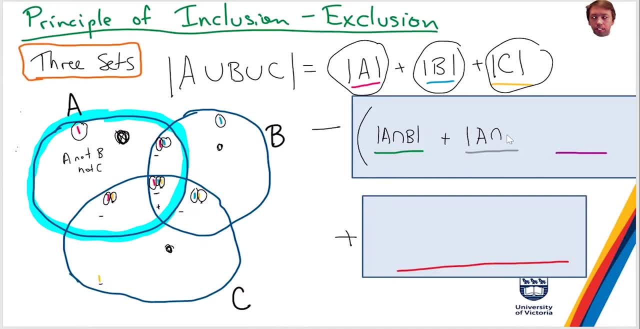 why this is going to work you know right now, But we'll see why it works And then I'm going to do this at the end And then I'll kind of try to explain this in more generality, why it works. 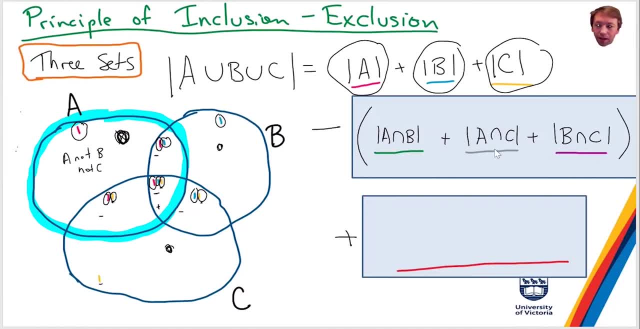 But yeah, what if I now subtract A intersect B, A intersect C, B intersect C. So when I subtract A intersect B, I subtract everything. everything here gets- oops, not there, that's A intersect C. everything here gets subtracted once. everything here gets subtracted once. Is that clear? Because? 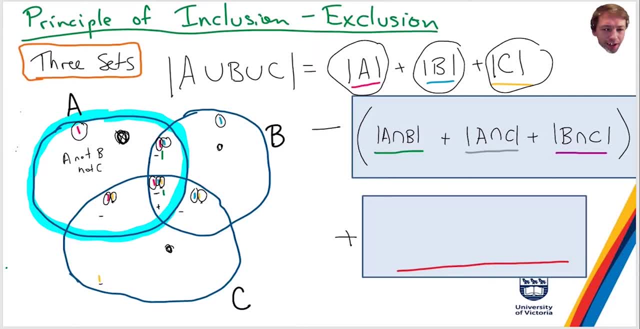 I'm A intersect B is this segment Right? I assume you can see my cursor right. But yeah, A intersect B is this segment here, And so everything's getting subtracted once in this green thing. Okay, I know this is a little. 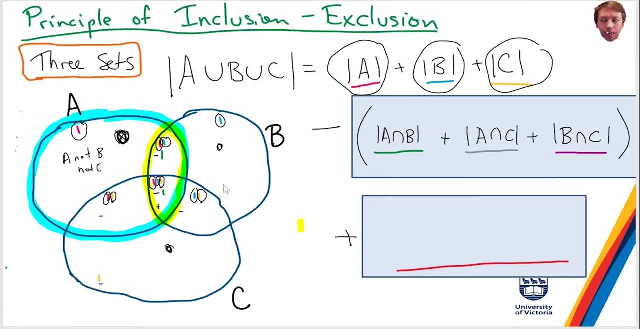 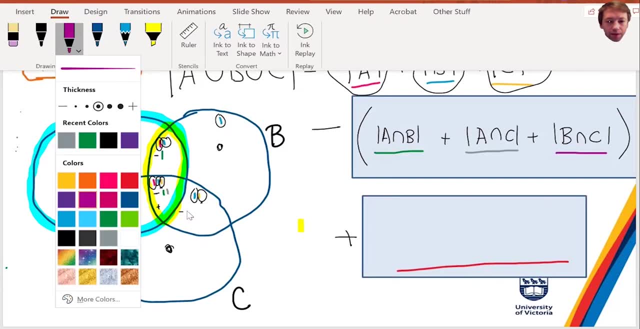 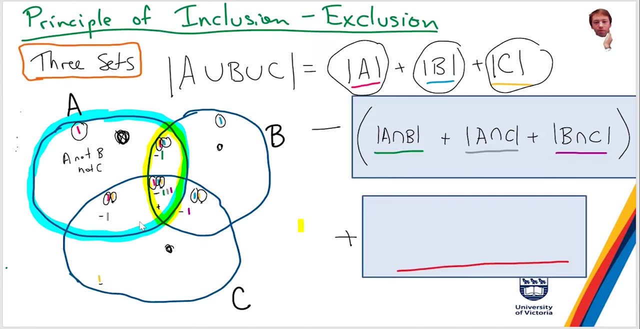 bit boring, But when I subtract A intersect C, I subtract everything here once. Okay. when I subtract B intersect C, I you know, everything here goes down by one right. So if you look at the situation we're in now, it actually looks like we're almost. 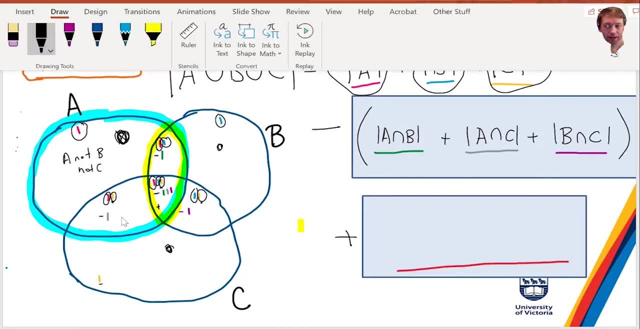 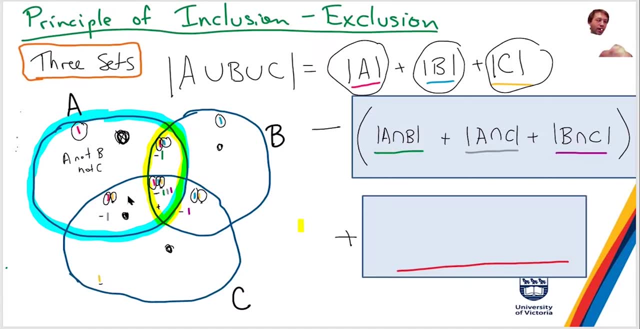 happy because actually here in you know, this area, I added everything twice, which is bad, But then I subtracted it once. So if I added it twice and subtracted it once, I've only counted it once. So, like at this point, you know, everything here is good, Everything here is good, Everything here. 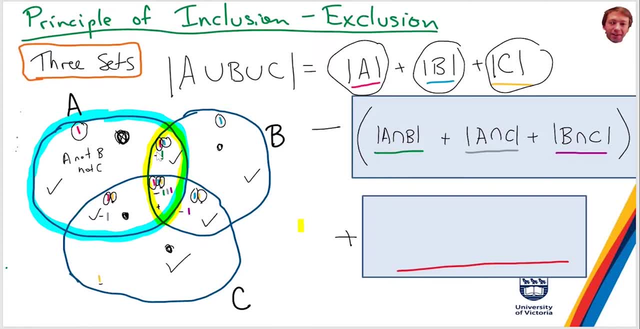 is good And here's good. Here is good, Here is good Because, you know, I either counted it just once or counted it twice and then subtracted once. But here is the very center is bad, And here is the very center is bad Because I've counted it three times And then I subtracted three. 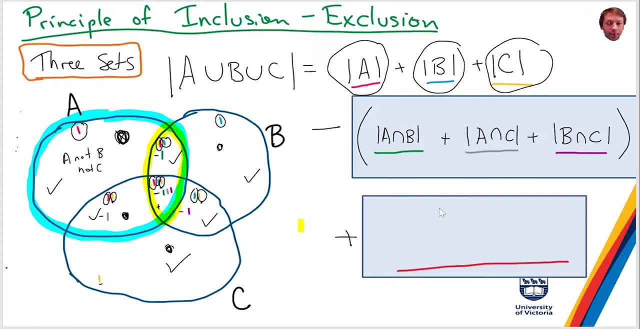 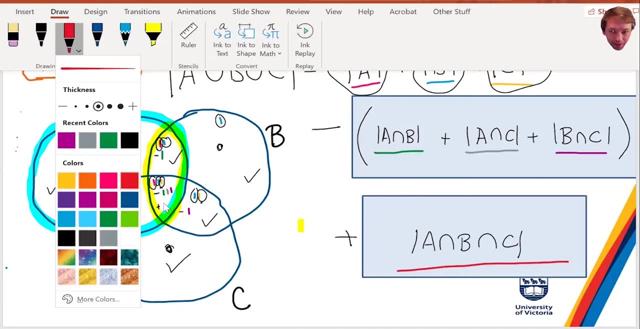 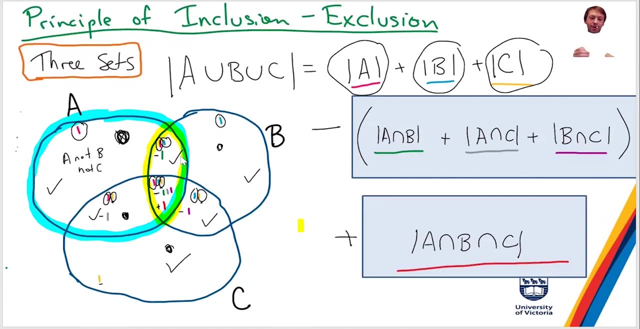 times. So I've actually counted it zero times. But then to the rescue comes A intersect B, intersect C. I add that on, And now I've counted that once. Okay, I'm not sure if this, this picture is kind of getting a little bit ugly, But if you look at like how many times everything was added, 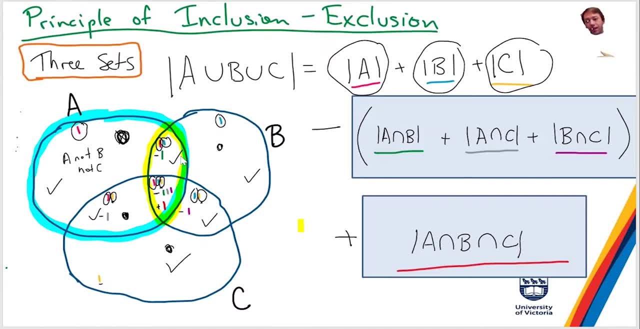 and subtracted, you'll see that in the end, everything gets counted exactly one time. Okay, this is a formula that you should really try to remember. If you are counting the union of three sets- A, union B, union C- the cardinality is: so: you take the. you know you take just one set at a. 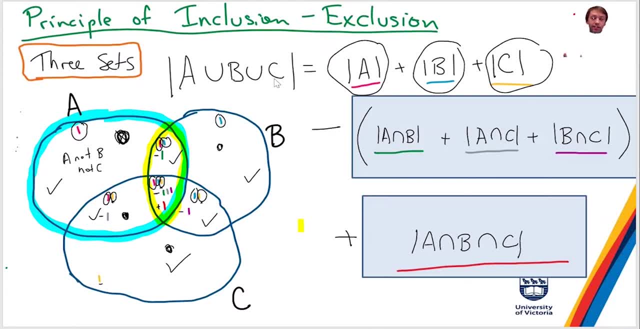 time A, B, C. you add up the sizes, you subtract the intersection of pairs of sets, So A intersect B, A intersect C, B intersect C. and then you add the intersection of everything, So A intersect B intersect C. Okay, And yeah, the reason it counts everything once. 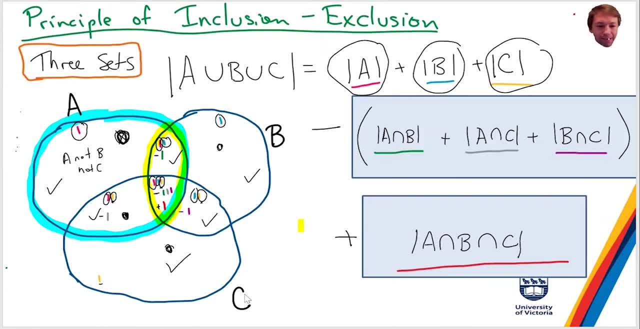 is because of this picture, Is that clear? Or Yeah? So, but yeah, so, like everything in this course, like I've mentioned a few times, you can either just memorize the formula or, like it's usually going to be more valuable, to understand the reason for the formula. But 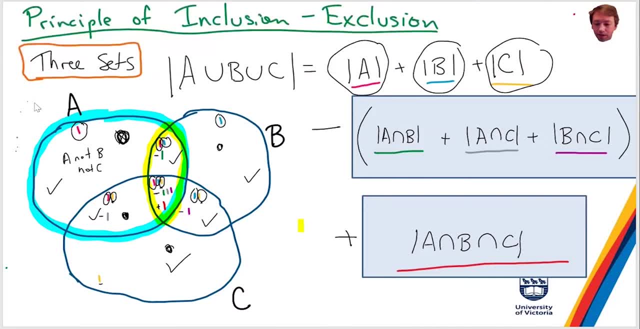 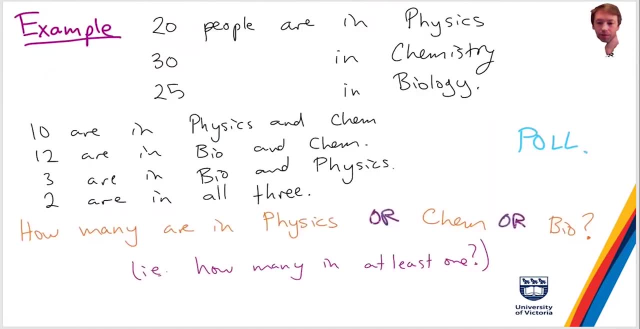 um, but yeah, understanding the formula is is going to be good as well for most questions. Okay, so let's do an example. Maybe I'll put this to a poll. So I apologize, it's kind of a long example to read, But I've got 20 students in physics, 30 in chemistry, 25 in biology, 10 are 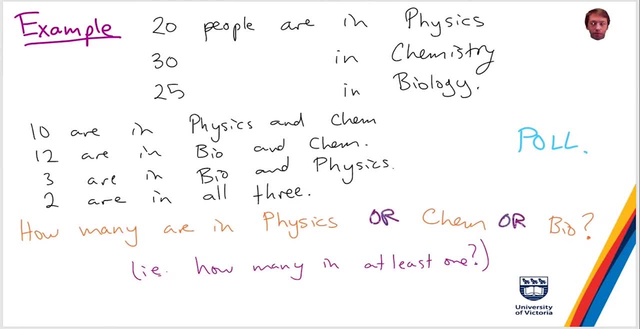 in both physics and chemistry. 12 are in both biology and chemistry And of course you know most biology students don't like physics. So only three are in biology and chemistry, And then there's two very keen people who are in actually all three subjects. So how many are in? 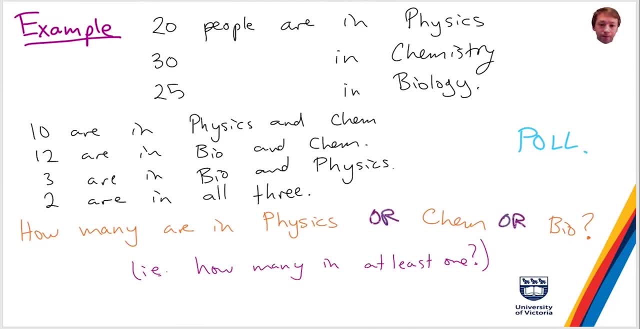 physics or biology or chemistry. Meaning, basically, if I took all the students from all the classes, I put them in a room and I counted them, how many would I have Right? So looks like people are understanding this one. I'll start solving it And then I'll 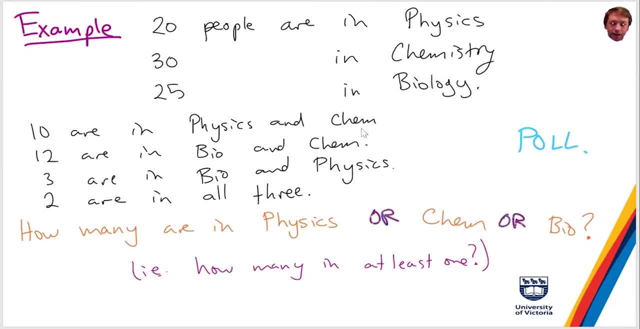 close the poll. But indeed, like the answer is, you know, you add them all up, So 20 plus 30 plus 25, you subtract the intersection of the pairs of sets, So you subtract 10, which are, in physics and chemistry, 12, and three, and then you add two. 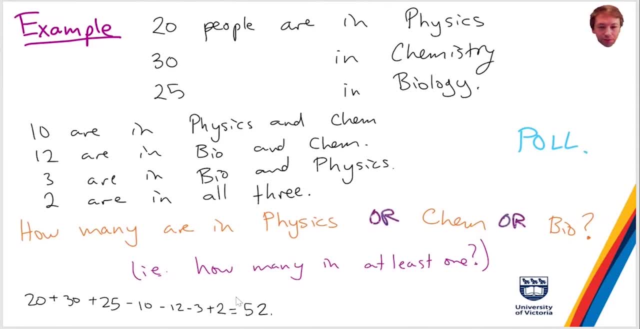 which, if I did the math correct, is 52.. Okay, And if you wanted to formally apply the, the formula we had before, like you can let a be the set of all physics students and so on and so forth. like, B is the set of. 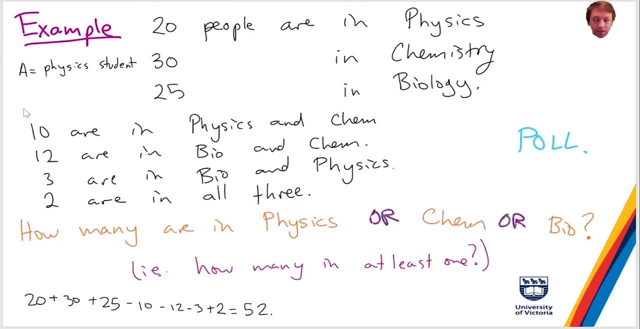 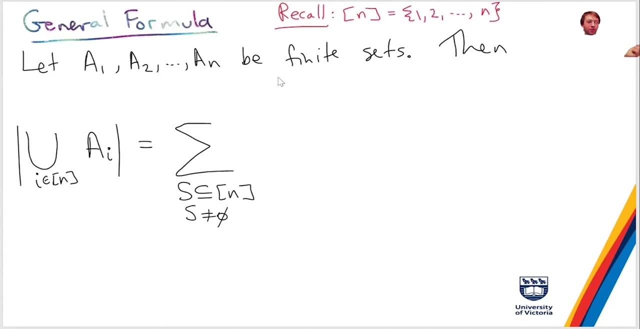 Chemistry students and C is a set of biology students, and then you can just apply the formula: Okay. so looks like everyone who Submitted an answer actually got the right one this time. Okay, Okay. so I assume that this is fairly clear. this is the, the part which. 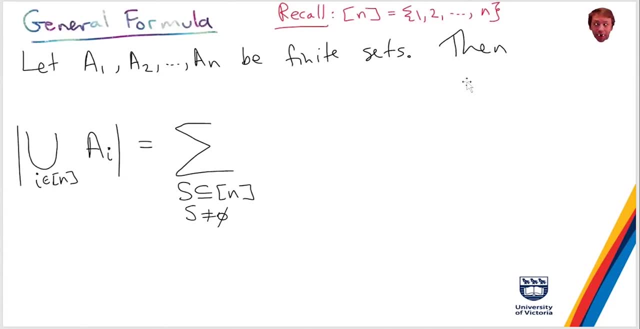 so Might be a little bit harder to grasp because it's like a little bit abstract. But now I want to give you like the general formula for inclusion, exclusion. So, by the way, everything, the stuff that I'm talking about, this thing where you take, you take all the sets, you add them up, you subtract the. 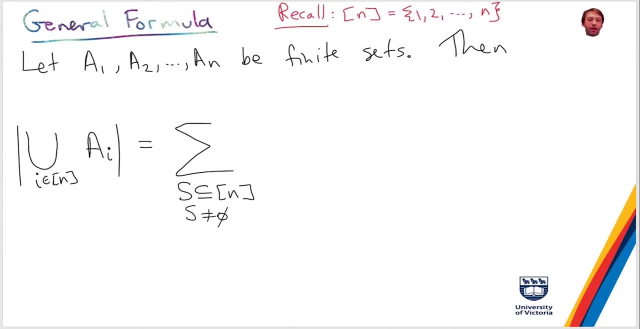 Intersections, add the three-way intersections, blah, blah blah. That's called the principle of inclusion, exclusion, Okay so. so what's the general formula? So, if I take so here, we've done two sets, We've done three sets, Like I want to give you. 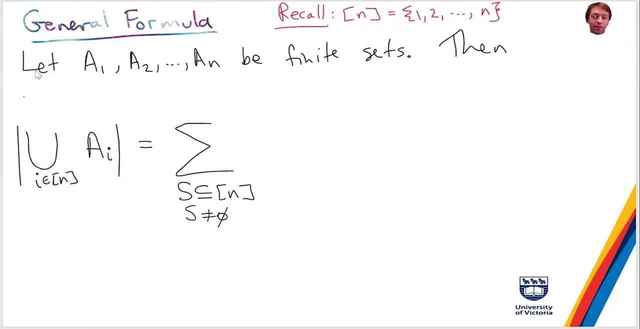 A formula now that will work, no matter how many sets I take, right? So if I take a hundred sets and I want to say how big is the Union, This is going to be a formula that gives the answer. Okay, Now, part of the difficulty here is going to be understanding what the formula says. 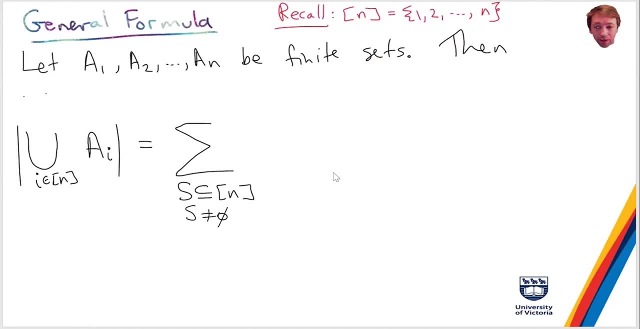 Because I'm gonna write it in very kind of formal, like abstract, kind of mathematical notation. So please do ask questions Or slow me down, But so recall, so I'm. So this is something we I mentioned a long time ago, but we don't usually use this notation. So 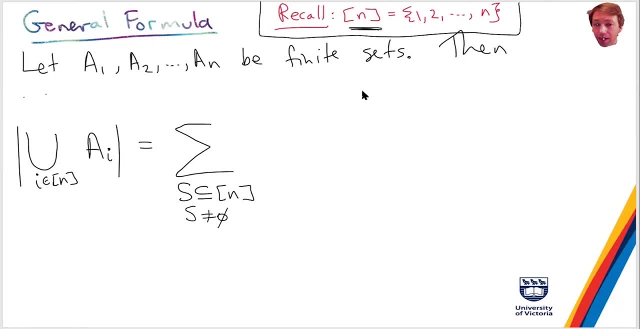 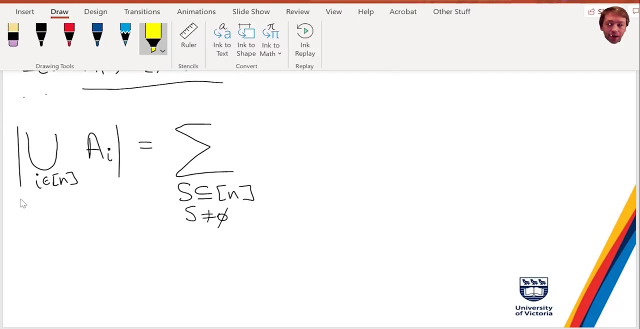 let's say square brackets. n is the first n integers and I let a 1 up to a n be a bunch of sets. then I want like, so, for example, if before we had three sets, so n was equal to 3, and I want to have a formula for how big the Union is and 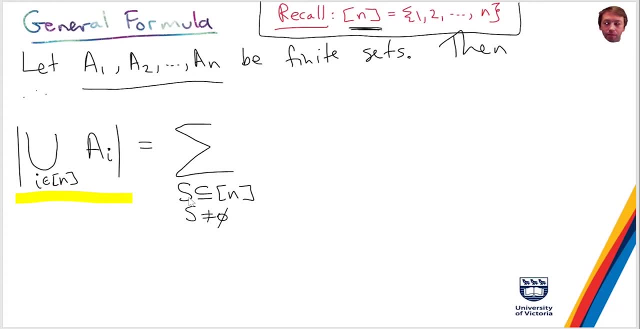 The formula goes like this: So you add up, so the index set is all the subsets of 1 up to n which are not empty, okay, and What you want to compute here is negative 1 to the size of s, plus 1 times the intersection. 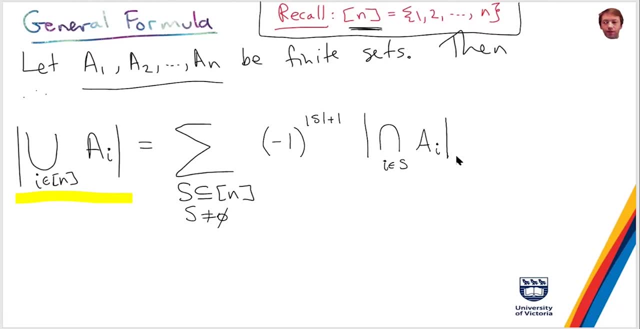 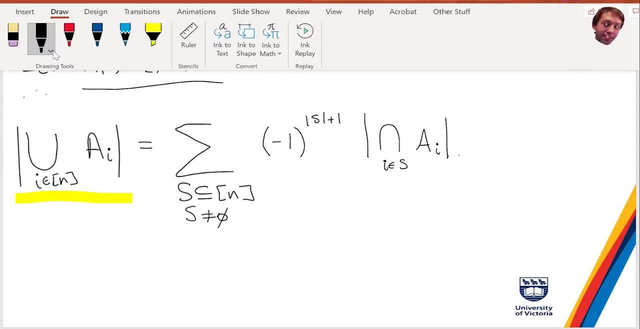 overall I and s AI. if you think about it, this is the same as This is. well, this is a generalization of what we've been doing for two and three sets. right, Let's look at the case of three sets and, like, try to understand what this says. 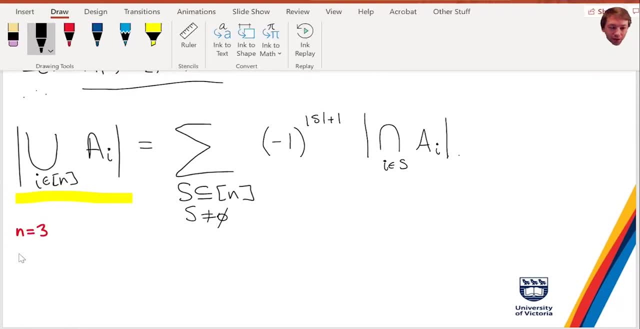 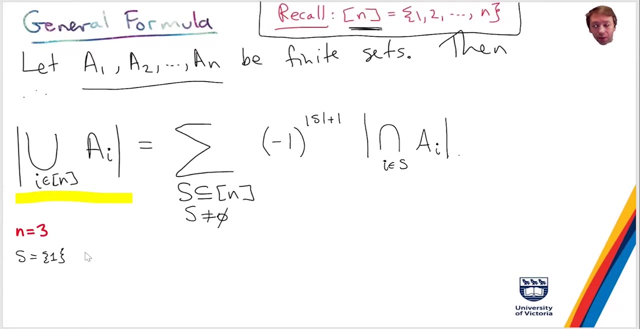 Like suppose n is 3, right? So if I take the term like, so we're gonna add up for every subset of 1 up to n, except for the empty set. we have a term of this sum. so the term corresponding to s equals 1 or s equals the set containing 1 is just the size of a 1. 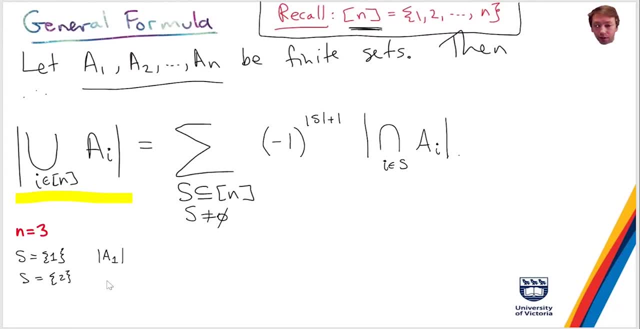 right, and s equals the set containing 2. you get the size of a 2 because, yeah, because, because, like say, if s is one like this, the intersection over all i and one of a, i or a, yeah, a i is just equal to a1. so that's where i get this thing okay. and here we have negative one. 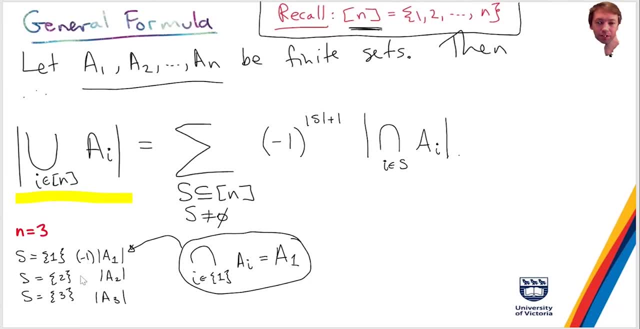 we also have this negative one to the size of s plus one, which is two, so, um. so let's not forget that. okay, is it clear what i'm even what i'm doing right now? i'm just trying to explain this formula in a. in the special case, n equals three, um, right, just to show that it's. it is in fact the. 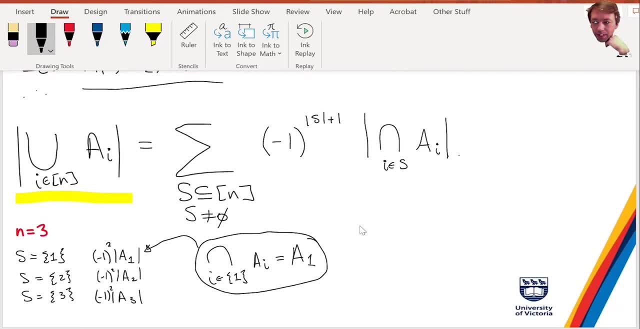 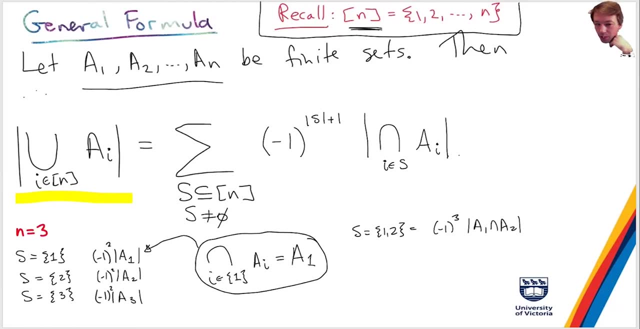 same as what we've been doing. so when i have the set s equals one, two, you get negative one to the three. a1 intersect a2 and of course, like negative one, squared is just one right. that's the kind of point here, that like that's just one. 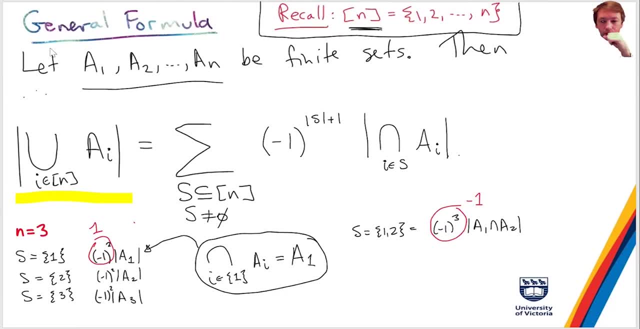 and this is negative. 1 cubed is just negative 1. right s equals 1, 3. you get. well, I'll just write negative a 1, intersect a 3, because negative 1 to the 3 is negative. 1 s equals 2, 3. you get negative a 2 a 3 and then s equals 1, 2. 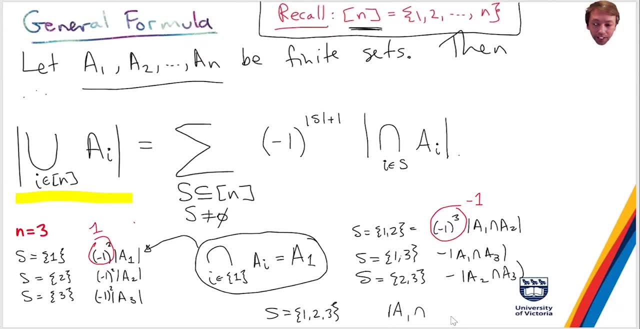 3, you get the intersection of everything: a 1 intersect a 2 intersect a 3, and so you can see that the inclusion exclusion gives us the the same formula we got before, right, you add up a 1 plus a 2 plus a 3. subtract a 1 intersect a 2. a 1: 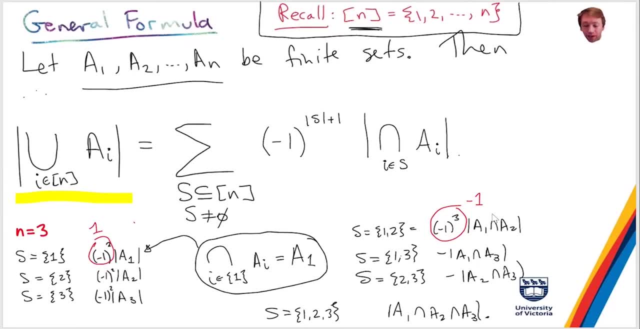 intersect a 3. a 1 interest a 2 intersect a 3, and then you add up, add in. yeah, so this is negative 1 to the 4, which is 1, the intersection of all three. okay, so from this you can also get a formula: when you have four sets, right, when you 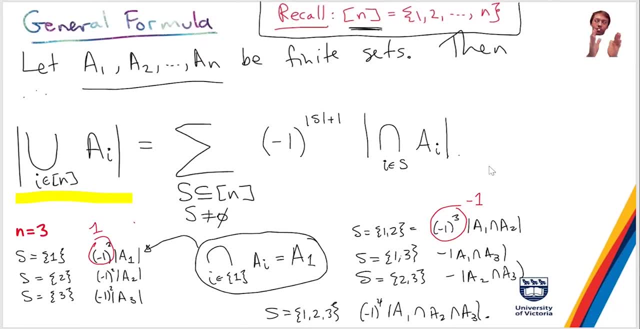 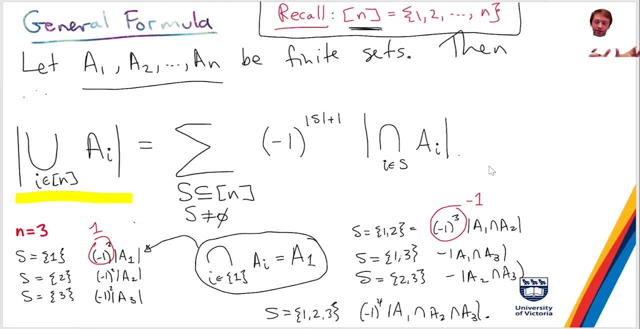 up the size of all four sets. subtract the pairwise intersections, like the first set, interests like the second, first interesting third versus just like fourth and so on, and then you're gonna add in the three-way intersections and then you're gonna subtract the four-way intersection. okay. 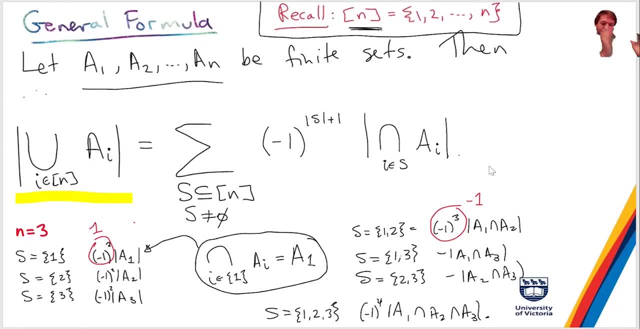 so it's just like an alternating sum, right? you take things of, you know, one set at a time, two sets at a time, you subtract them. three, you add four, you subtract, five, you add six, you subtract, and so on and so forth. okay, is this clear. okay, i'm going to assume that nothing in the chat and and general 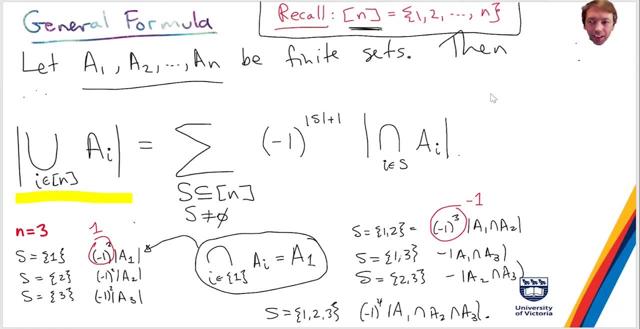 silence means that it is at least somewhat clear. um, but, like i said, uh, so this stuff, like understanding this stuff today is going to be important on thursday. um, so, yeah, so don't think that this is going to go away. um, inclusion, exclusion is going to be used again on thursday. 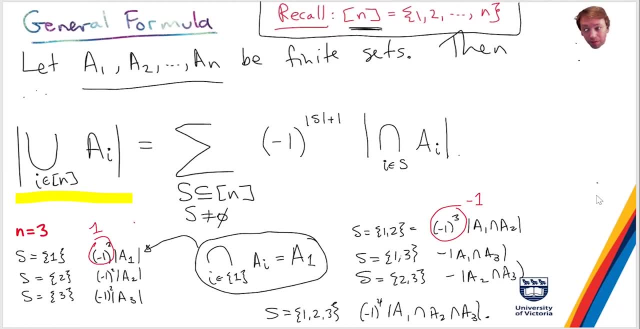 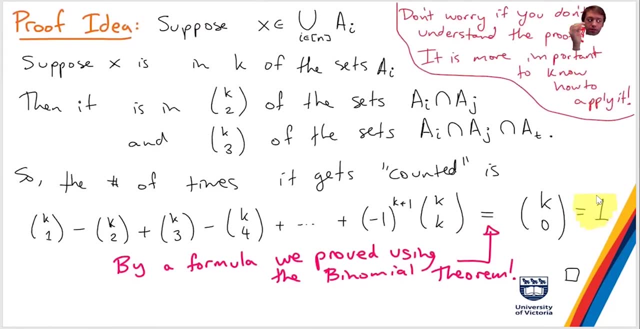 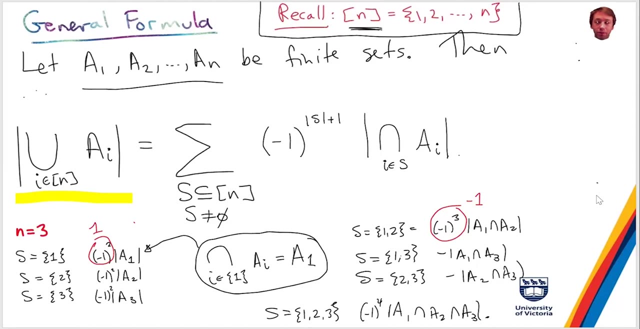 to prove some, uh, general results, some, well, to to prove some interesting, um, counting results, okay, so, yeah, so i've got this formula right, let's give. so i'm going to give you, um, well, basically i'm going to give you a proof of this formula. okay, so you don't like? i, i want to kind. 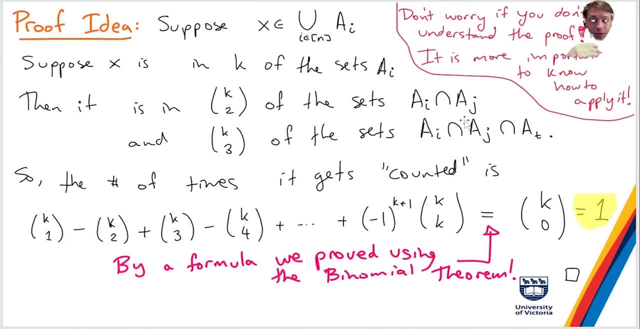 of stress that you don't necessarily need to fully understand this proof, like it's more important to know how to use the formula than to know how to prove it. so i'm going to give you a proof of this, um, but if you do understand this proof, it might- you know, it might- be kind of valuable for you in. 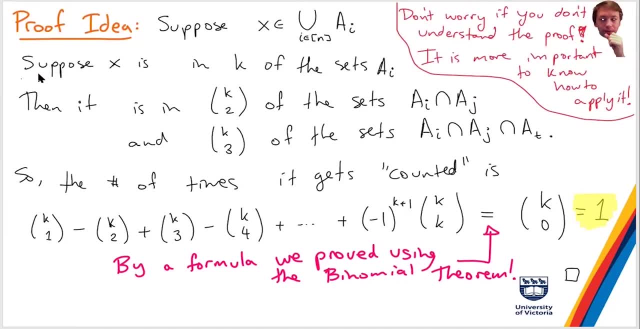 some cases, right, um, but anyway. so i'm going to give you a proof. if you don't, uh, if you don't understand it, then don't worry too much. but okay, so i want to count the size of this union. right, i've got sets a1 up to an. i want to say how big is the union. so suppose i have a set, a point an. 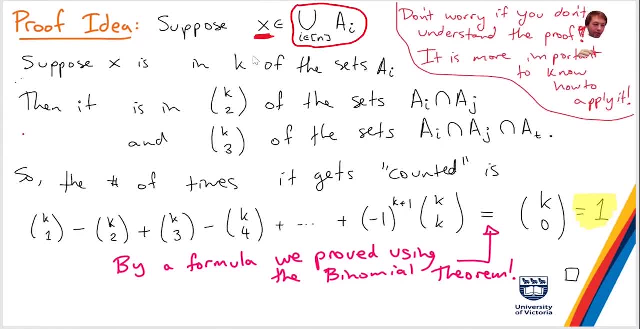 element x of the union. so i want to count. basically, i want to count x exactly one time, right, i want to count everything in the union exactly one time. so what i want to check is this. so, if i take the formula that i wrote out, the question i want to ask myself is: how many times was x counted? okay, and 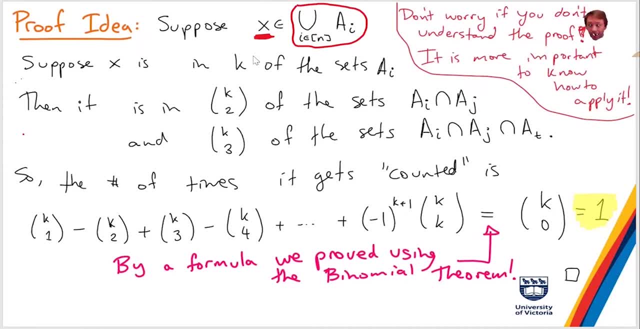 if the answer is one, then that's awesome, because i want every element to be counted once, but i have to show that it's counted exactly one time, okay. so how do i do that? so i'm going to give you a proof that. so i assume that x is contained in k of the sets a, i where k is at least one right. so i, i want. 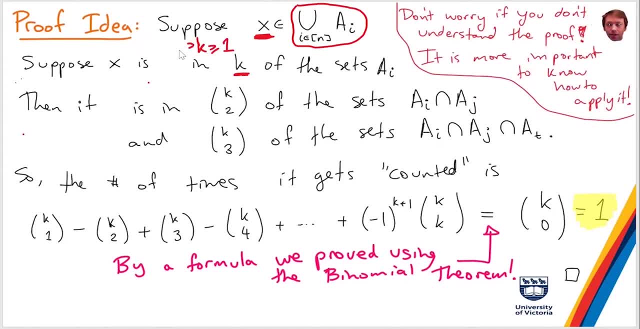 to do this in generality, right? so k is at least one and at most n, right? i want to do this in complete generality, so like if x is in exactly one of the sets, or if it's in two of the sets or three of the. 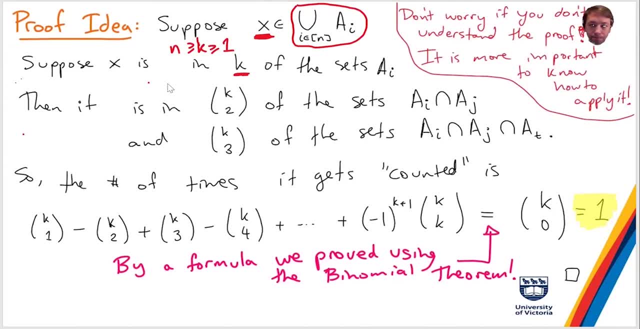 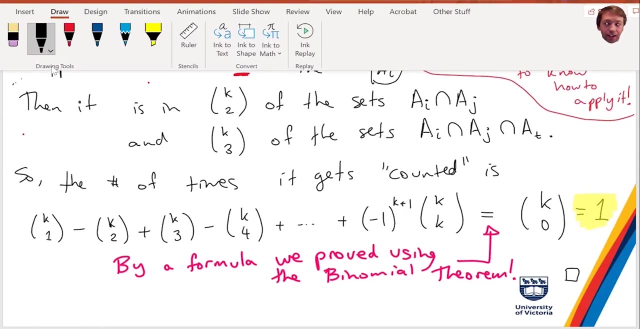 sets. i want it to uh to get the right answer. um, so, how many? so like. what i would like to ask now is that x is in k of the sets a, i, how many pairs of indices i and j are there? so, how many or how many? 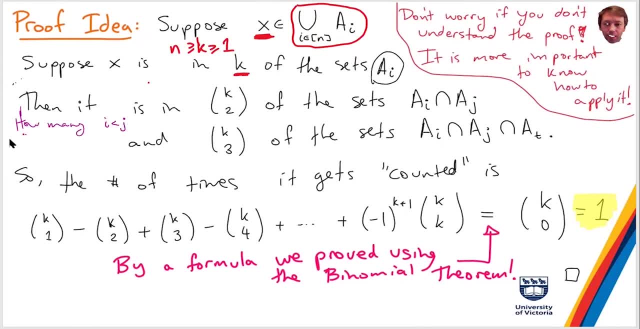 yeah, indices i where i is less than j, let's say, are there such that? sorry i'm writing this in a little nook and cranny here, but uh, um, how many pairs of indices are there? where x is in a, i intersect a j and i've already given the answer here. but if you think about it it's not hard to. 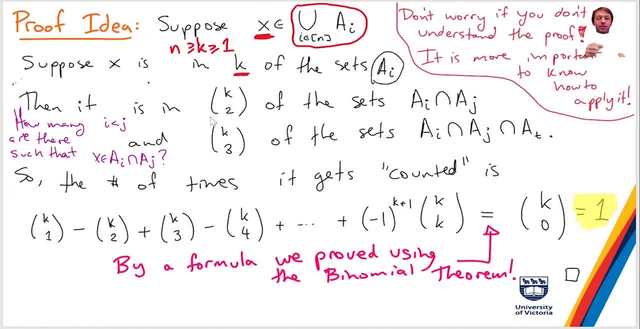 see that it's k choose 2 right, because in order for x to be an, a i intersect a j. x has to be inside of a i and in a j and the number of ways to choose so and there's k things that x is in. 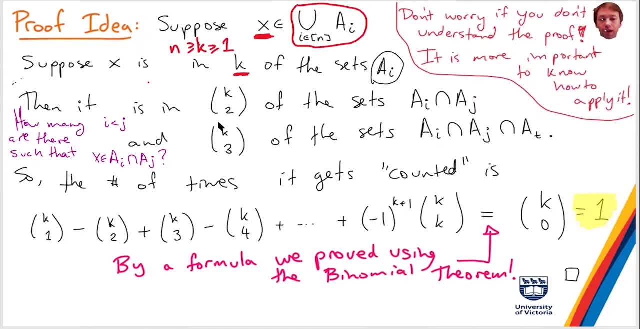 so the number of ways to choose two of them is: k choose 2 right and and then, similarly, x is is contained in k choose 3 of the sets: a 1 intersect, or sorry, a i intersect, a j intersect a t, where i, j and t are distinct. 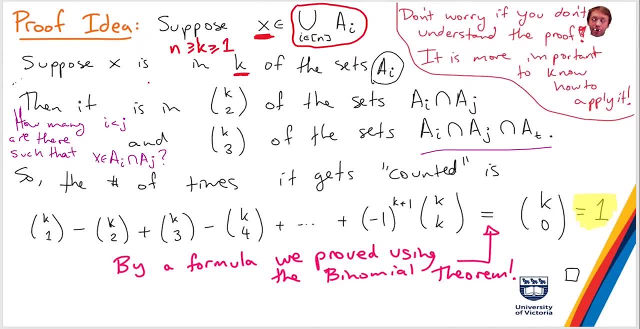 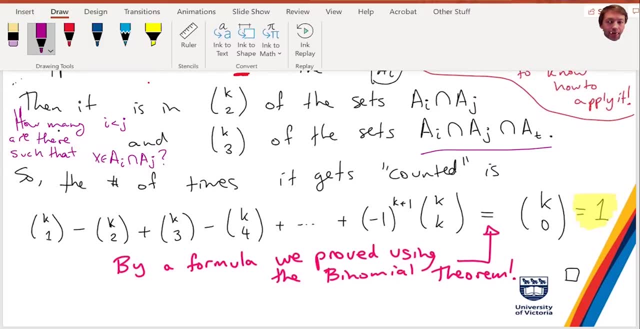 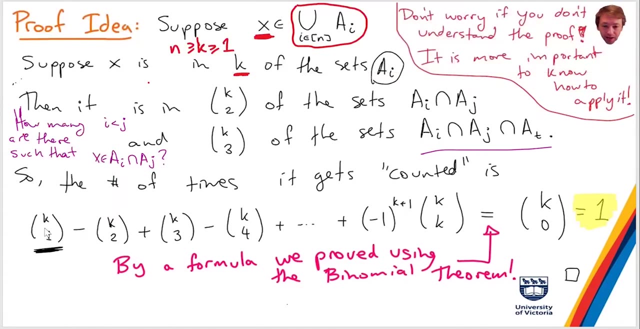 so we, yeah, can actually determine immediately how many times X gets counted by the formula, So the number of times X gets counted. so when I take the sum of the size of AI that's gonna count like X gets counted K times. K choose 1 times, but K choose 1. 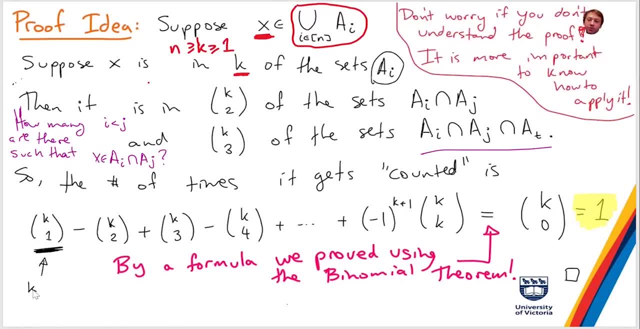 is just K, because X is in K of the sets, When I subtract the pairs, the size of the pairs of the sets. sorry, the intersection, yeah, these intersections, AI, intersect, AJ, I'm gonna subtract K, choose 2.. Like in terms of: 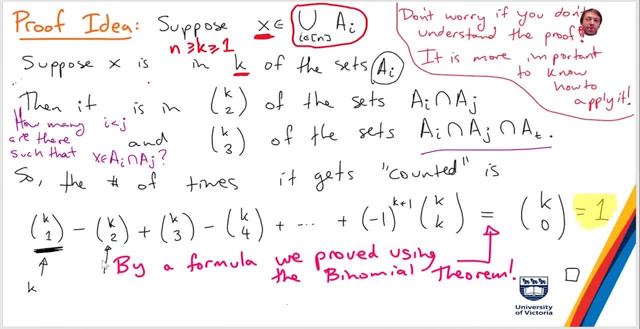 I'll you know that'll count X, K, choose 2 times and I subtract it in the formula so I get a minus K, choose 2, plus K, choose 3, minus K, choose 4, all the way up to plus or minus K, choose K and actually one of the. so this, this is actually. 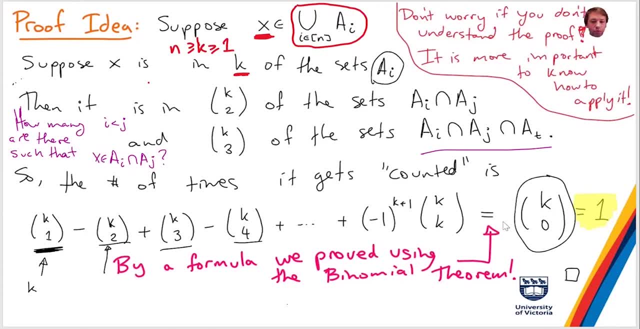 equal to K, choose 0. Which is 1.. And that follows from one of the formulas we proved with the binomial theorem. right, Remember we, if you take, if you take X plus Y to the N right Binomial theorem says that this is N choose K from K equals 0, or maybe I'll 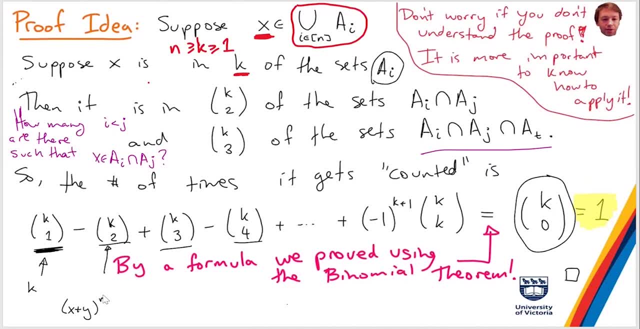 maybe I shouldn't use K here, I'll use. I'll use K in the exponent So X, choose, X plus Y to the K is the sum of I equals 0 up to K, K choose 1.. K, choose I, X to the I, Y to the N minus I. And remember in the thing on the 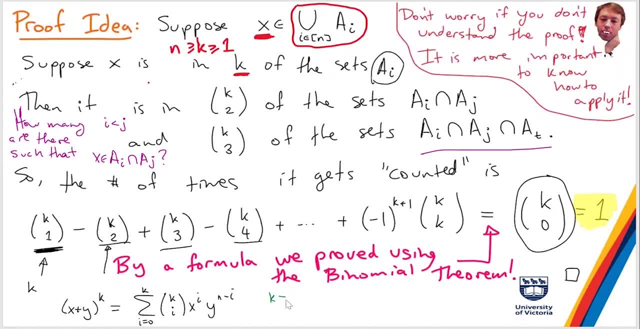 binomial theorem. if K is at least 1, which it is right, We all already assumed- K is at least 1.. We can set: X equals 1.. Y equals negative 1.. And the left-hand side is just 0 and the right-hand side is the alternating sum of binomial. 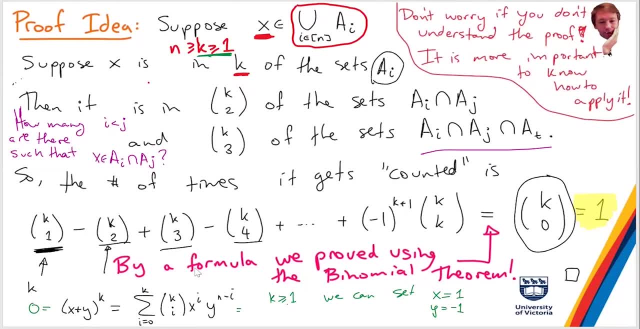 coefficients. So yeah, so. So then you get this, this formula, Okay. so I know that that was a bit, maybe a bit abstract and a bit quick, but are there any questions about this proof? Like I said, if you understand the proof, that's great. If not understanding the, 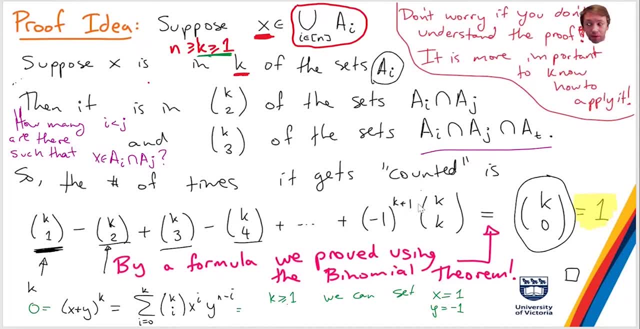 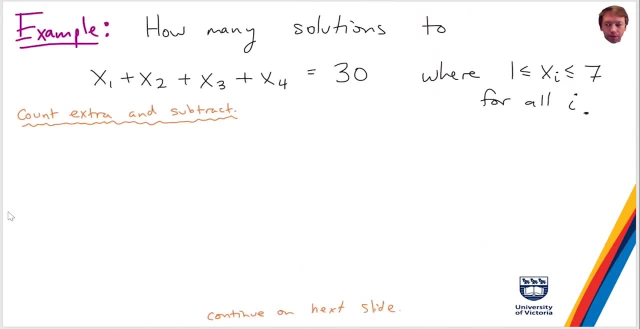 inclusion-exclusion formula is the most important part of this, But are there any questions about the proof? Okay, So let's maybe play with the with a few more examples. So here's an example of something which is kind of similar to some questions we've already seen. 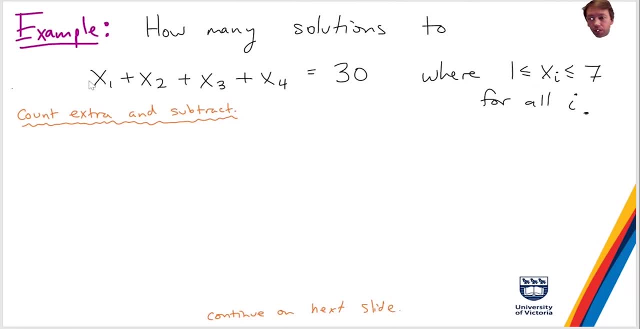 but there's a bit of a twist, right. So remember these questions where you say I want to count integer solutions to x1 plus x2 plus x3 plus x4 is 30, where. so usually in these questions we've mostly dealt with like: 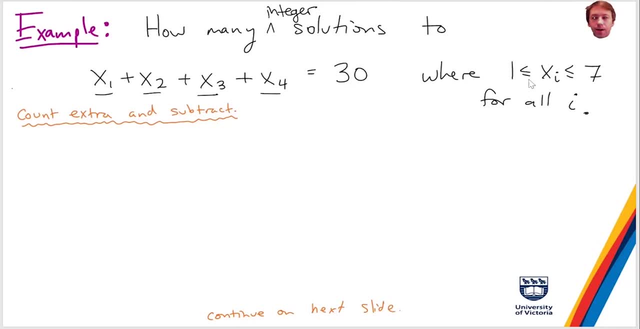 a lower bound, So xi is at least one. Occasionally I've thrown in, like at most, seven on one of the variables. But here we're going to deal with, like, all of the variables have an upper bound of seven and a lower bound of one. 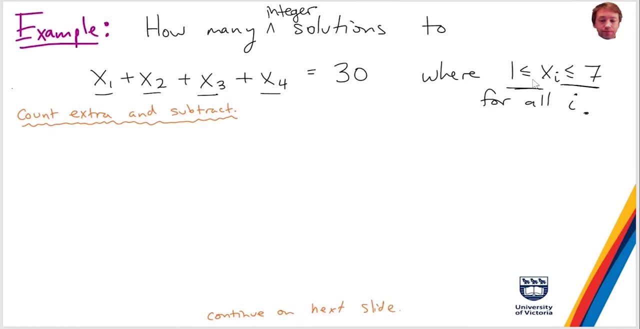 So all the variables are between one and seven. So how can we solve this using inclusion-exclusion? Any ideas? I hope it's not zero, Is that, Oh dear? Okay, let's change the question a little bit. It is indeed zero. 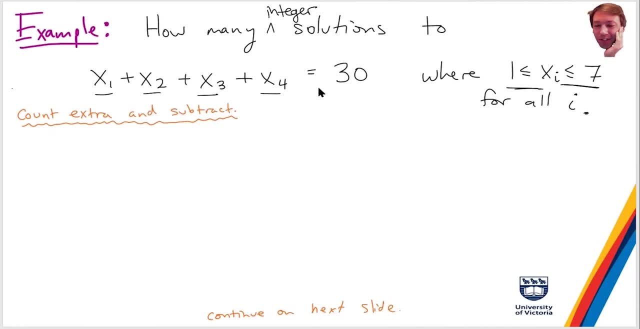 How silly is that. If I add up four numbers, which are at most seven, how big can they be? They can be 28 at most. Yeah, that was rather silly. Let's change this a little bit. Let's make it nine. 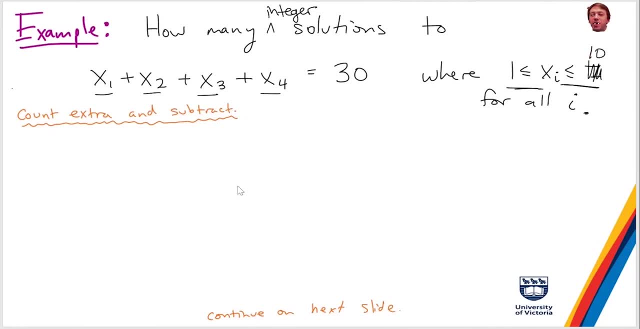 Let's make it 10.. Okay, Okay, The question was broken. Let's, so now it's fixed. Okay, So now the answer is not zero, but good point. So how many ways can we do it? Okay, Well, so, rather than like, 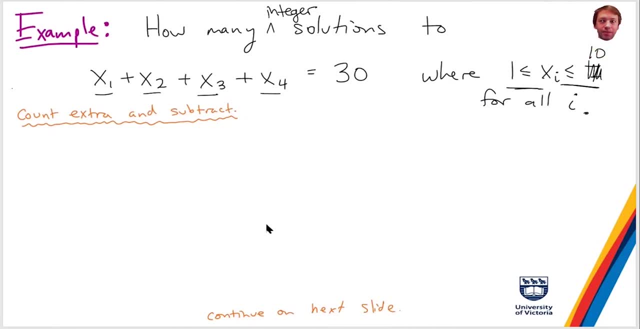 I don't want the final answer at this point, but you know what's the concept here, right? So, and the hint is to count extra and then subtract. right, Let me see what's on the next slide. Yeah, So. so how would I? 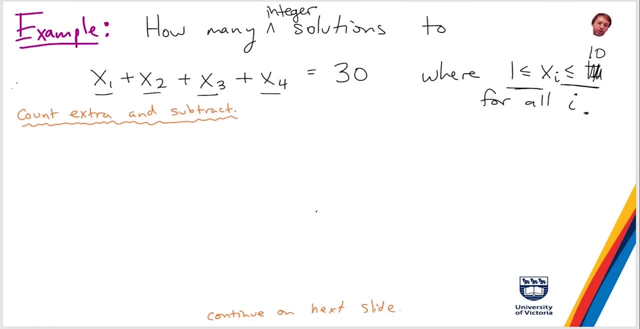 how would I do that? So what I'm going to do is I'm going to first just count solutions where xi is at least one, and then I'm going to count. there's no restriction, no, like upper bound restriction, Like so, in other words, 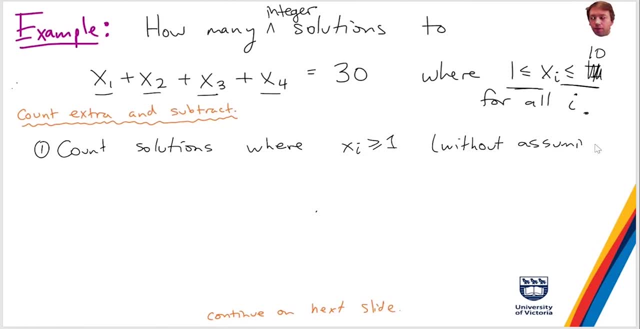 without assuming, assuming, without assuming- that it's at most 10,, right, And if I count all of those solutions, that's going to be too much. right? I don't, because some, some of them will have the thing going above 10,. 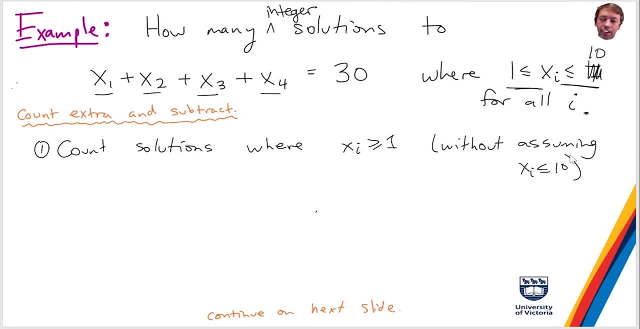 but then I need to subtract the ones that I don't want. Okay, So how many solutions are there to this sub problem? So, where we just assume xi is at least one, Does anyone remember how to do these? So xi is at least one. 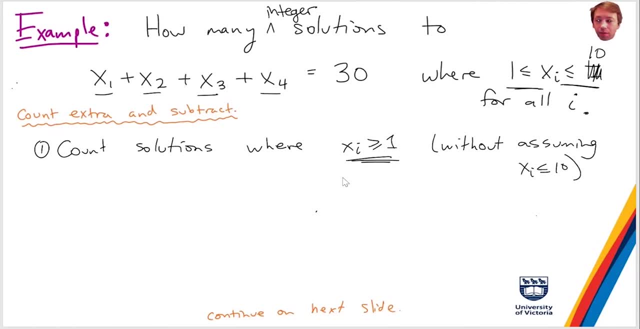 How many ways can I add x1, x2, x3, x4 to equal 30? Any anyone remember this? So this is from probably, yeah, the second week of classes or something. Yeah, Okay, So we've got the. 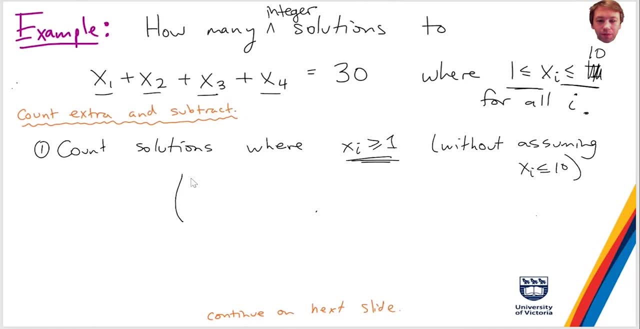 we've got the, the answer coming in in the in the chat. right, So it is indeed 29,. choose three. The way to think of that is: you can take, you know, 30 identical balls or something, and then you have 29 different gaps between them. 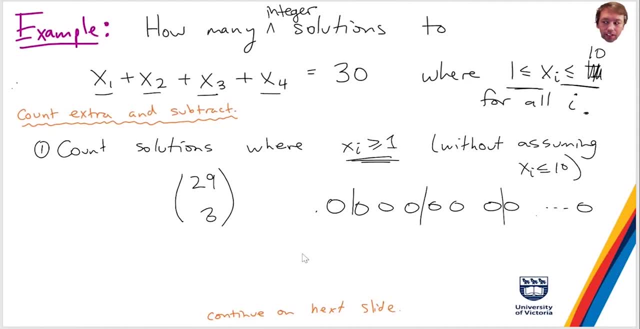 And then you're going to choose three of them, right, And x1 will be how many balls you have in the first group, X2 will be how many you have in the second group, and so on. Okay, So 29,, choose three. 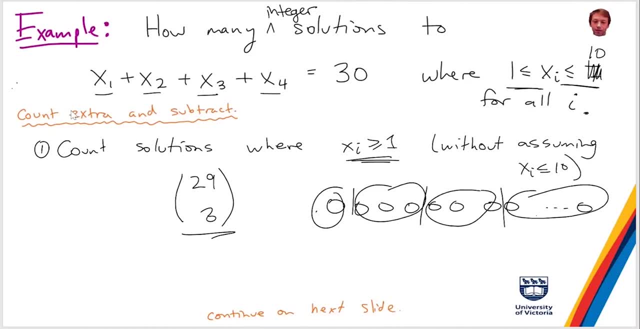 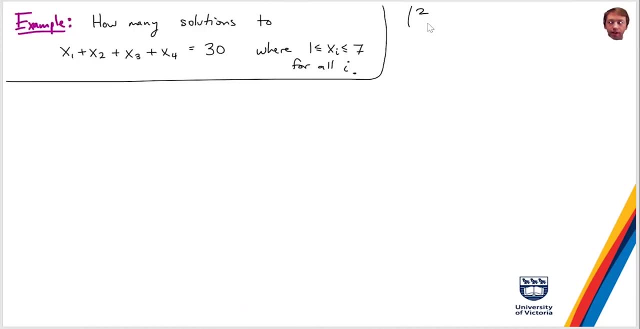 But now we need to subtract the solutions that we didn't want to count Right, So so we've got 29,. choose three solutions if we ignore the xi. So this is going to be at most 10, the xi at most 10 condition. 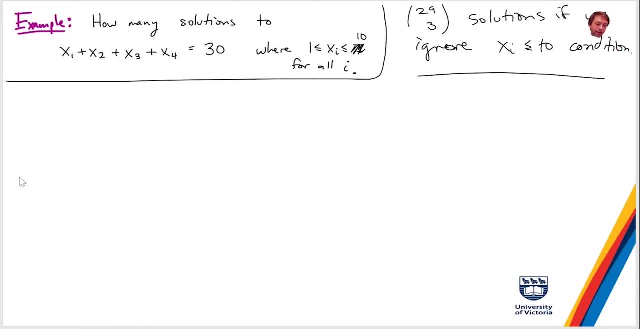 Okay. So how many of the solutions have one of the xi's greater than 10?? So let's say I'm going to say ai, let's say yeah, so for for i between one and four. so I'm going to do this kind of fairly formally, just yeah. 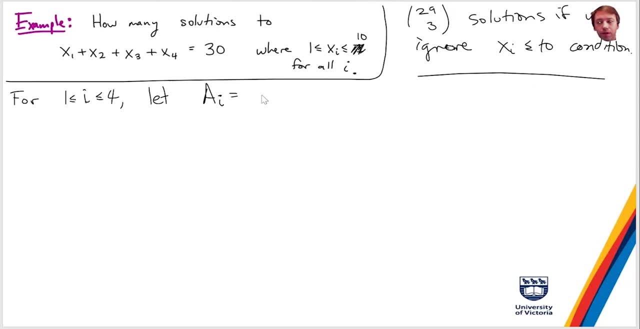 to kind of connect this to the, the formula. so I'll let xi be the, the set of all. well, okay, maybe the set of all x1, x2, x3, x4, such that xi is at least 11.. Oops, Okay. 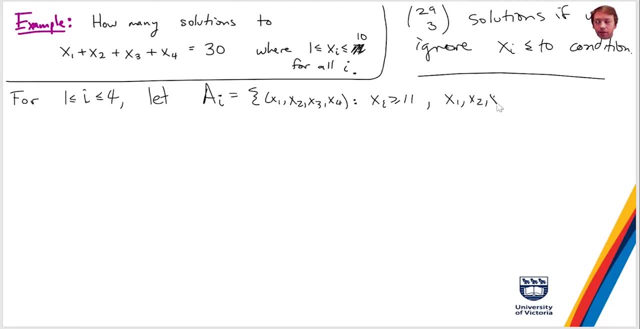 So you know all of the x, so this is going to be a bit redundant, but all of the x's are at least one and they add up to 30. So sorry if that's not that readable, but right. So I want to count the bad solutions. 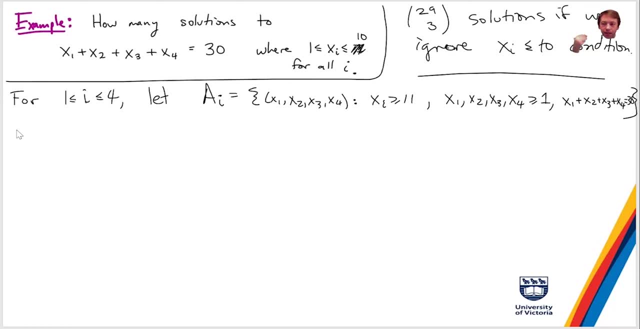 right. The bad solutions are the ones that have that property where somebody went above 11.. So what I want to count is a: a one union, a two union, a three union, a four union, a five union, a six union. 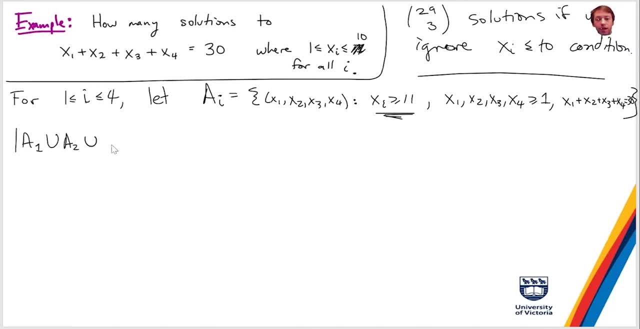 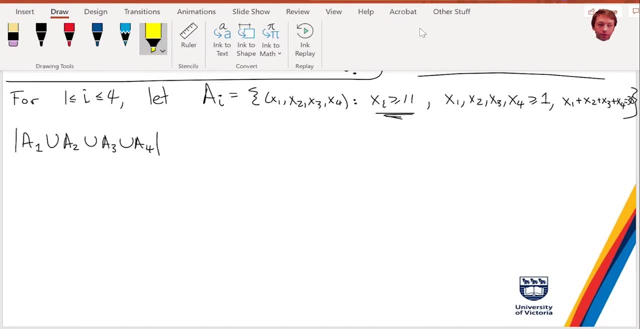 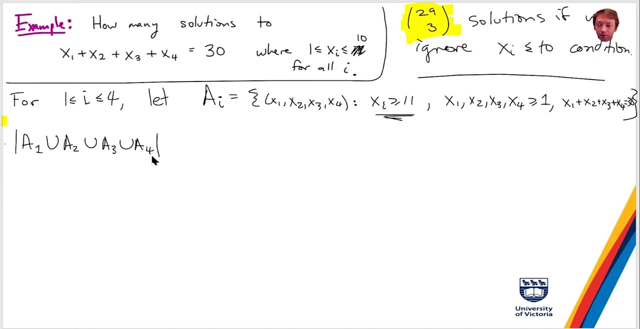 a seven union, a eight union, a nine union, a six union, a three union, a four right, And we want to subtract this from our first like solution thing, which was 29 choose three. So I want to take 29 choose three and I want to subtract whatever I get for this union. 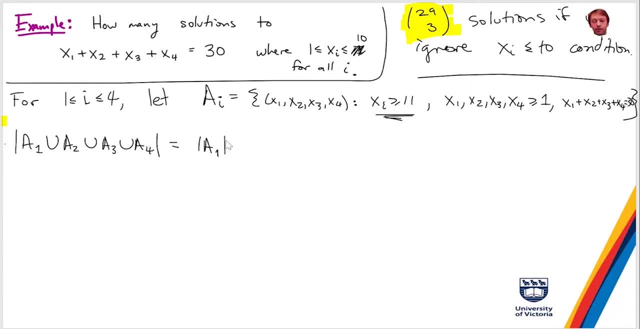 So well, so it's yeah, so it is equal to some big, you know sum by, by, inclusion, exclusion. Let me kind of think about, let's think about some specific terms of the sum, though. So how big is a one? 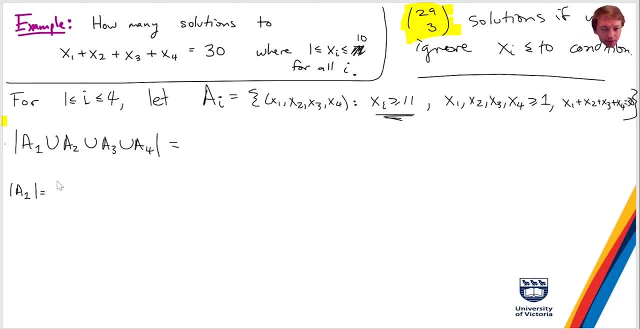 Any thoughts? So a one is the number of solution. The size of a one is the number of solutions. right Where x1 is at least 11 and x2 is at least one, x3 is at least one, x4 is at least one. 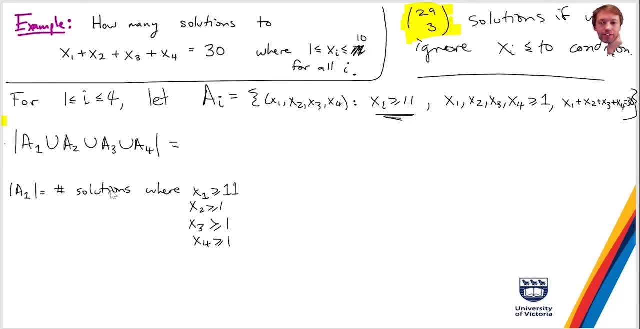 right. So does anyone remember how to do this? And yeah, there's no upper bound like constraint on the x size. Yeah, exactly, So we've got an answer, An answer coming in the chat of 19. choose three, which is correct, because it's kind of like. I first, because you can imagine you take out of your 30 things. 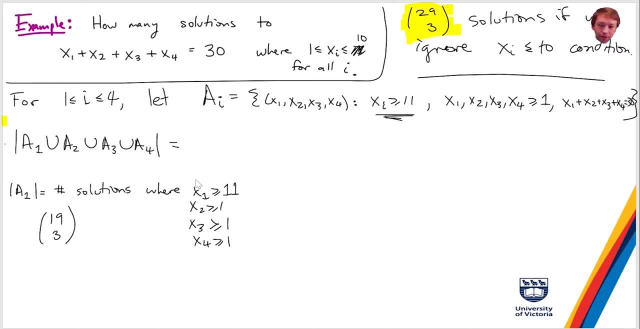 You can donate 10 of them to x1,, right? And then we're kind of just trying to divide up the rest so that everybody has at least one, and that's going to be 19. choose three, And then it's fairly clear, right, that if I take how big is a two? 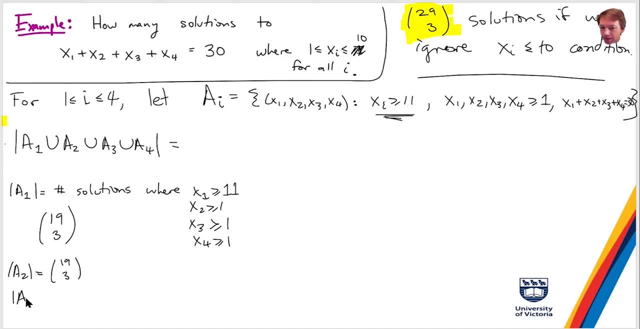 Well, that's also 19 choose three, right, So all of these things are 19 choose three. Well, because, because of the symmetry in this problem, So yeah, so, thanks for the participation, Right, Okay, so that kind of so. so the first kind of part of this sum is, like you add up, all of the size of a eyes. 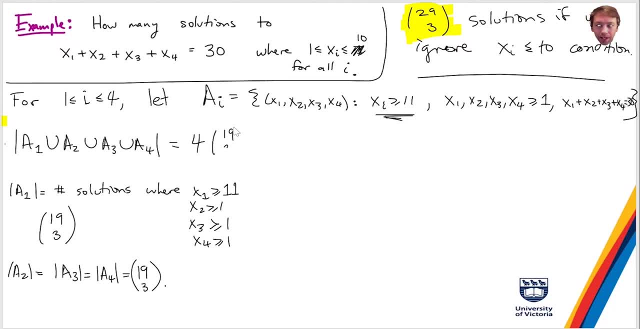 They're all 19 choose three. So we have four times 19 choose three. Okay, Now what if I look at how big is, Let's say, a1 intersect a2.. So does anyone have an answer for that? So that's the solutions where x1 is at least 11 and x2 is at least 11,. 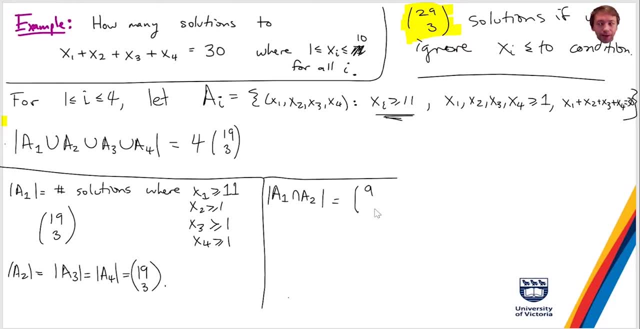 right. So if you think about it, that's going to be nine, choose three, because, yeah, I mean both of these you can think of with a substitution, right? So if you kind of: yeah, so this is like, you've got x1 at least 11, x2 at least 11, x3, at least one. 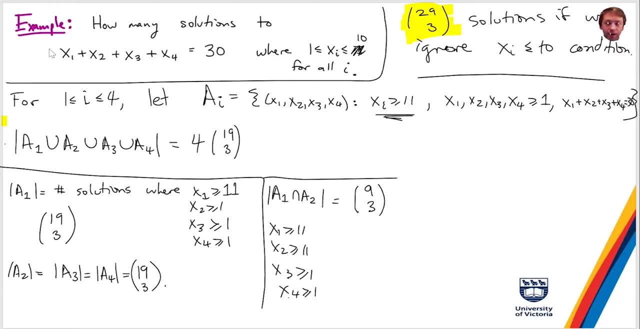 x4 at least one. you can do a substitution by. so you could have done the same thing in the first one as well, by just letting y1 equal x1 minus 10. y2 equals x2 minus 10, y3 equals x3, y4 equals x4, right. 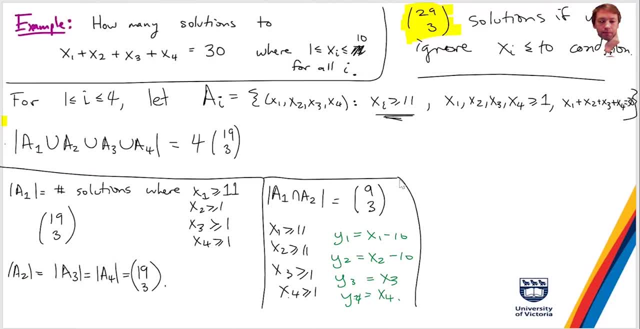 Anyway, and then, if you solve that problem, you're going to get nine, choose three. Okay, now, so then, yeah, so then this is going to be So: a1 intersect a3 is going to be the same size a1 intersect a4,. 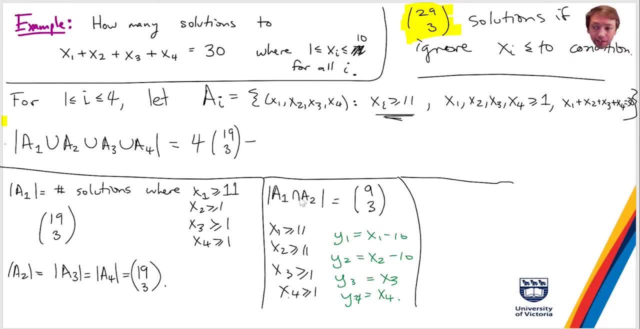 you know, all of the different pairs of sets- a1 and ai and aj have the same size. And how many of them are there? Well, there's four choose two. So four choose two times nine choose three. The four choose two comes from all the ways of picking one, like picking i and j from one to four. 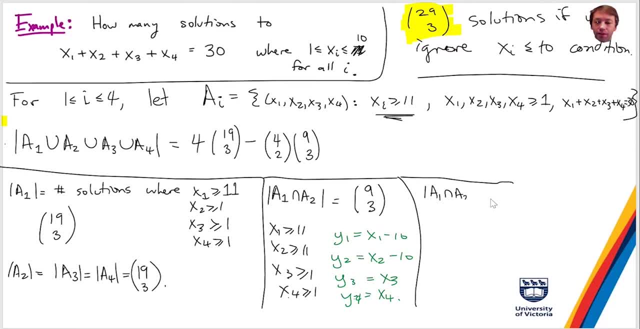 How big is a1 intersect a2, intersect a3?? And if you do that, you're going to get nine choose three. If you think about that, it's actually zero, because because if, if x1, it's kind of similar to well to how the question was kind of screwed up before- if x1 is at least 11, x2 is at least 11 and x3 is at least 11.. 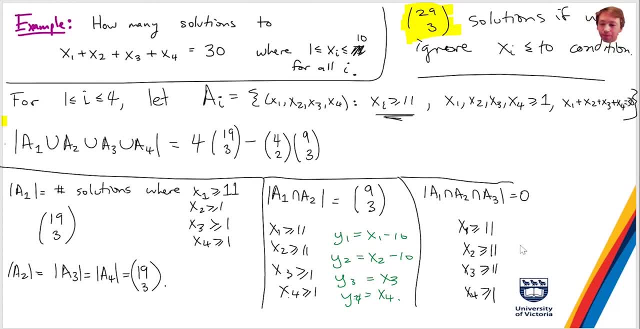 Well, we're already at an x4 is at least one. you know, we're already adding up to at least 34 the sum. So, in particular, it's impossible for this to equal 30.. Yeah, So then, actually, you know, 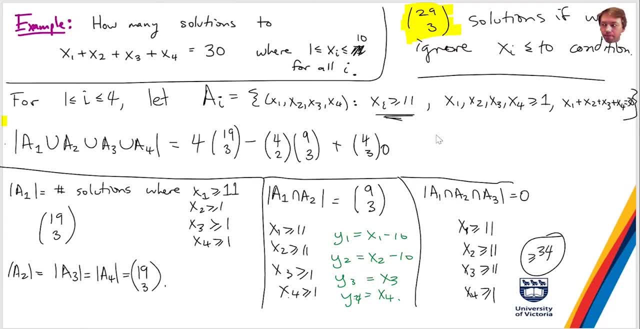 it's so. it's plus like four- choose three times zero, and then minus four- choose four times zero, because if I look at the intersection of all four of them, that's also empty. Okay, that's pretty much your legible there, but hopefully the idea is clear. 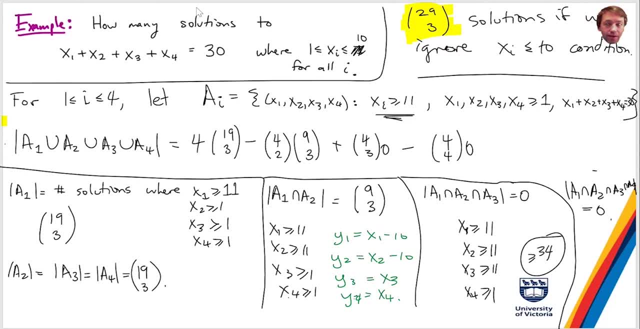 So the final answer, then, is: you take 29, choose three, which was all the solutions If you have no restriction, no upper bound restriction, minus the ones we didn't want Count, which is four times 19, choose three plus four. choose to nine, choose three. 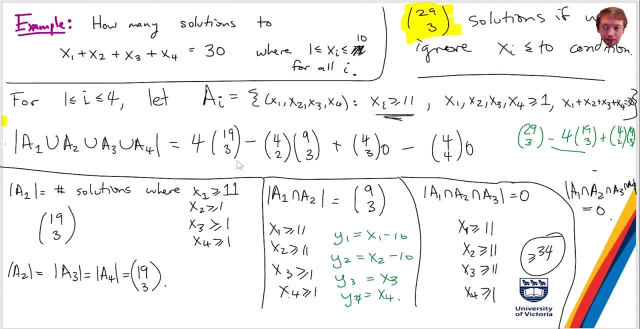 And this minus is because, yeah, we're, we're subtracting this and we're then we're subtracting this, which makes it a plus. Okay, so that's the final answer. Is there any questions about that? So this is kind of a combination of three different things we've learned. 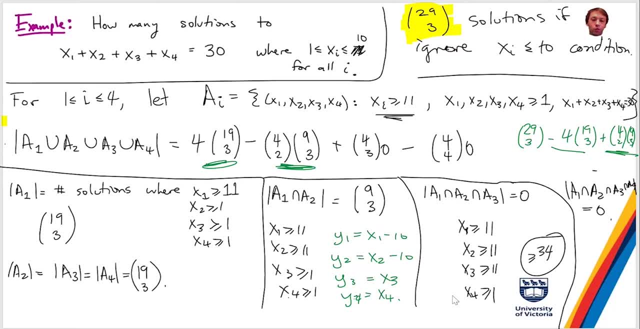 right. We've learned how to count integer solutions when you have, like you know, a lower bound restriction on the on the variables. So we've learned how to do that right, And we've learned how to count the complement right. 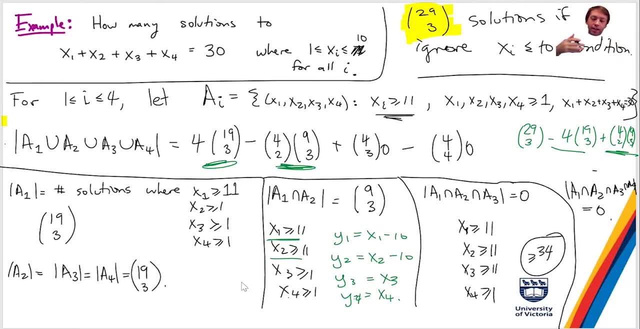 Counting the things you don't want to count and subtracting them, And then this is like also including inclusion, exclusion, So it's kind of a combination of lots of different things here. But yeah, you are supposed to, you are going to need to be able to combine lots of different things. 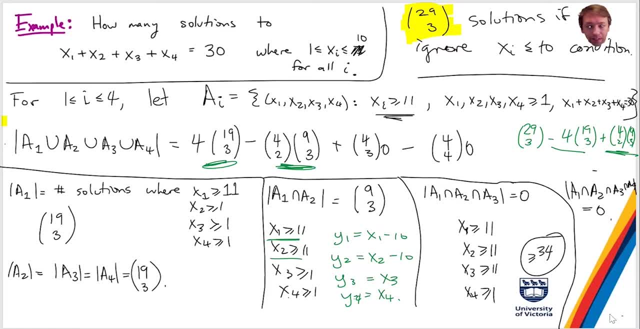 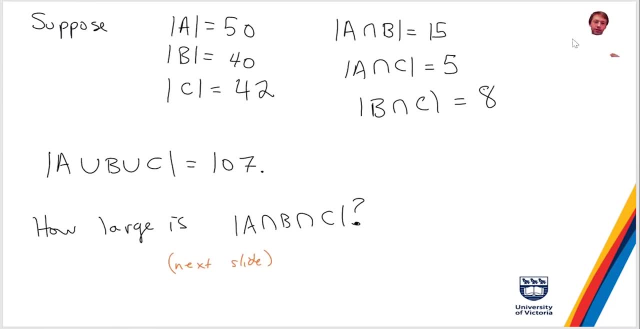 We've learned in different parts of the course. So this is good practice, Okay. so, um, here's the kind of yeah, here's a somewhat of a kind of reverse problem. So remember, like when in inclusion, exclusion, the formula I gave you is actually a formula for A, union B, union C. 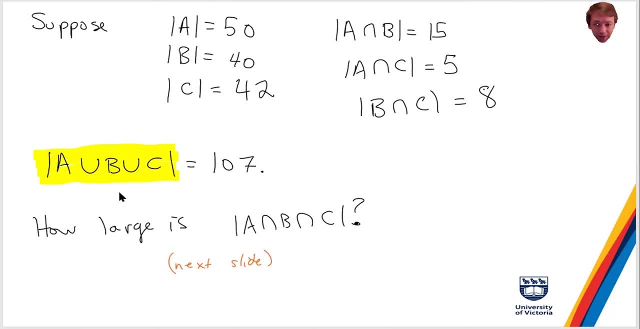 right. But let's suppose somebody gives you the answer to A, union B, union C, right, But they're asking for the intersection. So you have to be really careful in these questions whether like what they're asking for. you know, don't get the, don't get these two things mixed up. 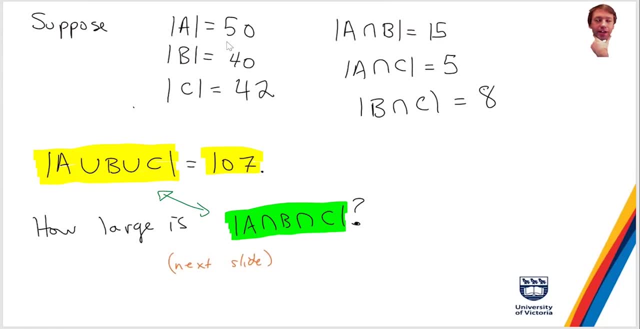 right, Yeah, so they. they tell you that A has size 50, B has size 40, C has size 42, the intersection of A and B is 15, A intersects C is 5,. B intersects C is 8,. 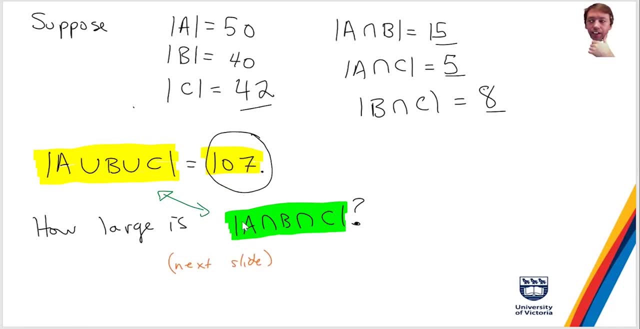 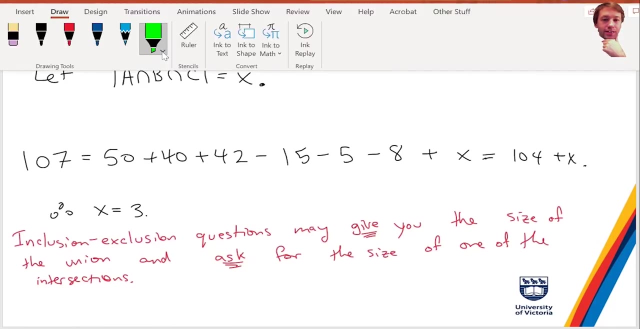 and they tell you that the union has size 107, and they want you to say how big is the intersection. Okay, but you can also get this from the formula right, Because just by kind of solving for the intersection. So let's suppose I let the intersection size like A, intersect B, intersect C. 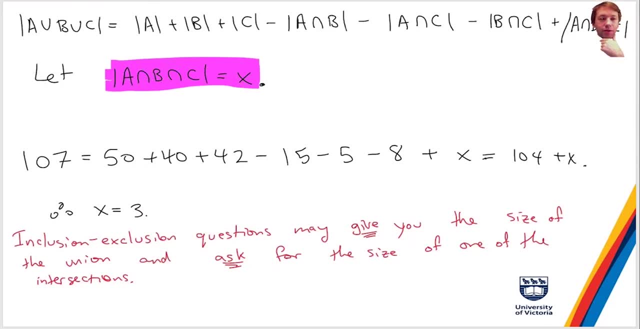 I let that be equal to X, right, And now we write down the formula. So what does the formula say? So it says A union B, union C is A plus B plus C, A intersect B, or sorry, minus A intersect B, minus A intersect C, minus B intersect C, plus the intersection of all of them. 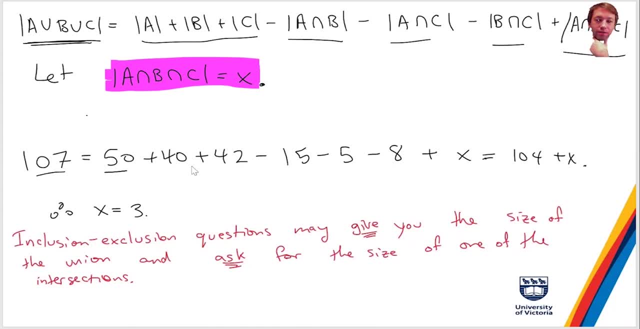 And you can just solve for X right. So 107 equals blah blah blah minus blah blah blah plus X right, Because X is equal to that, And so 107 is 104 plus X. Therefore, 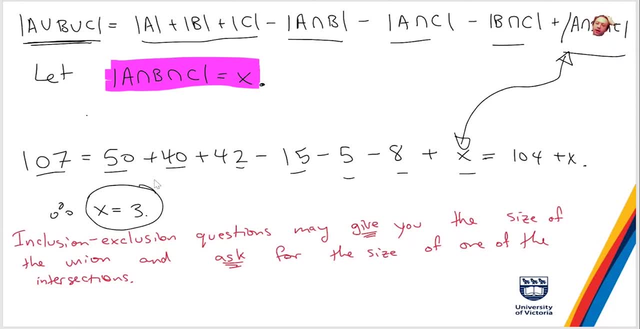 X is 3.. Okay, is it clear what I did here? So, in general, like you might not, in an inclusion, exclusion question, you might actually not be asked to compute the size of the union, You might be asked to compute something else. 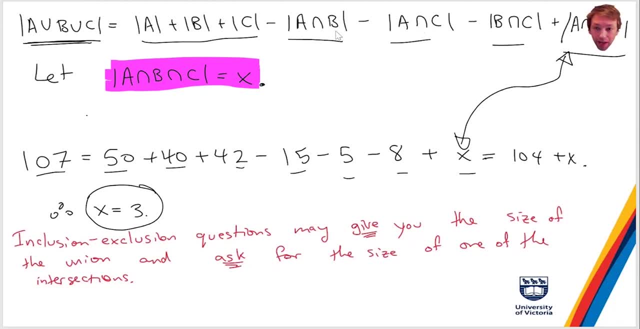 right, Like, for example, you might have been asked to compute A intersect B right, And so the important thing is to you know, to understand, that this formula can be used to compute any of these things as long as they give you the size of the union. 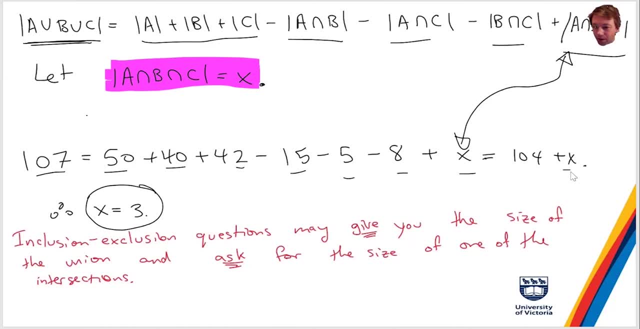 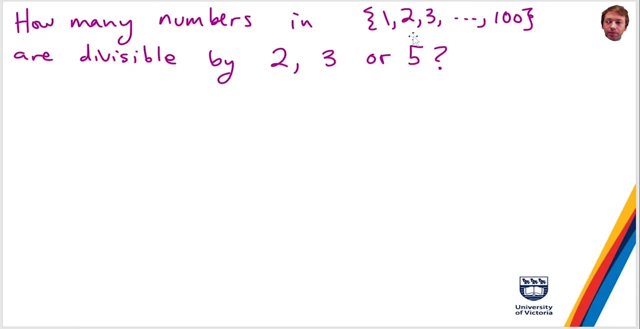 right, You can just put everything in, you know, write the thing you want as a variable. You don't really have to do that, but you can- and then solve for it, Okay. Okay, here's a nice example. How many numbers in the set 1 up to 100 are divisible by either 2 or 3 or 5?? 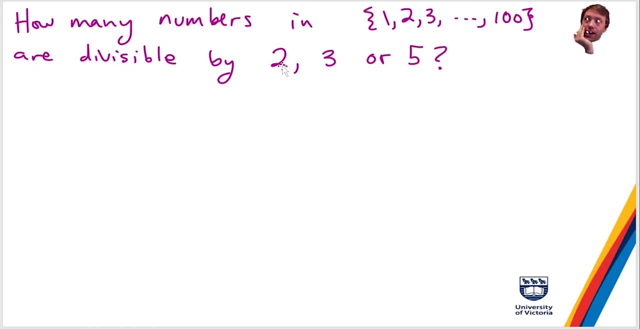 Okay, so actually just to connect to something. So remember, you know, remember back with the rule of the rule of sum. right, I told you that those are for questions that involve the word or. but there's also this tricky thing that it's questions that involve the word or. 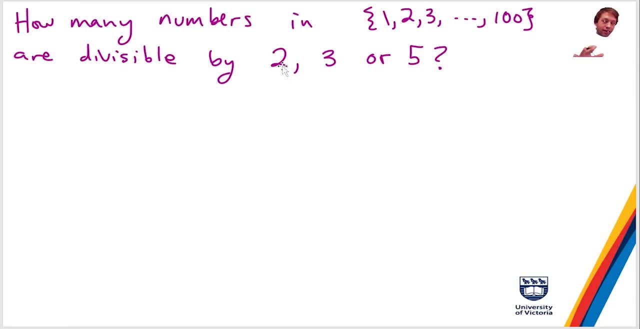 in the case when those things can't happen at the same time. Now, here, in inclusion, exclusion, when you're computing the size of the union, you know this word or is going to come up a lot, but here we have a situation where these things can occur at the same time. 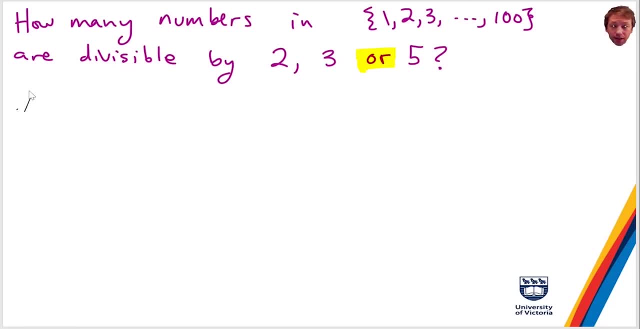 So okay, how are we going to do this? So let's say we let A2 be the numbers. Well, it's a set of all I in, 1 up to 100, such that 2, divides I. Does everyone know what I mean by divides? 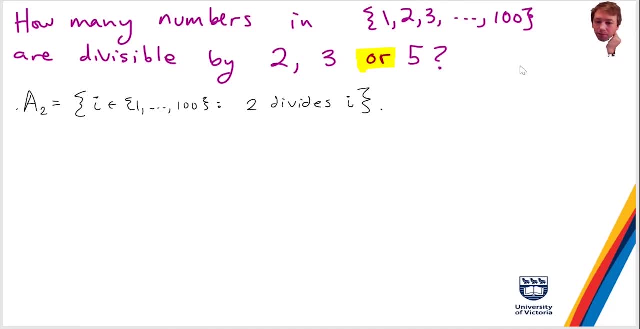 Like divide. when I say that a number is divisible by 2, it means that 2 divides evenly into that number. So, for example, you know, 5 divides 65, right, Because it goes in evenly. but 5 does not divide 66.. 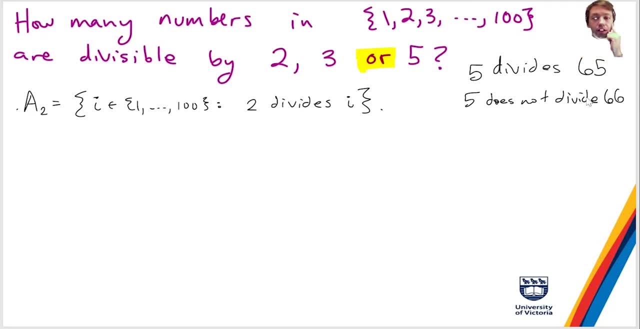 In other words, 66 is not divisible by 5, right And similar for 3 and 5.. So you know, 3 divides I and similar for A5.. Set of all I in 1 up to 100,. 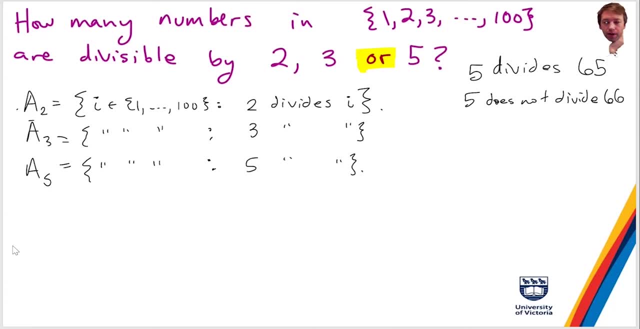 such that 5 divides I. So how big is A2? Any? so how many numbers between 1 and 100 are divisible by 2? Any answers: Exactly 50.. So if you think about it, but yeah, 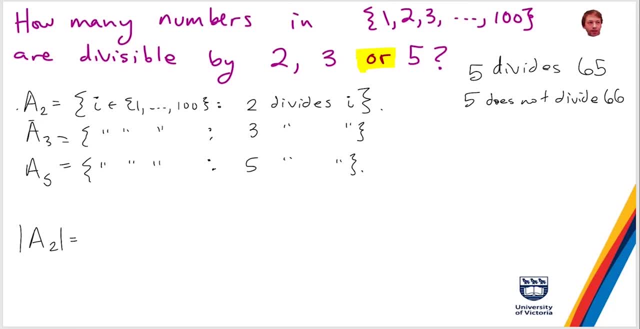 it's just all the even numbers, right? So it's 2,, 4,, 6, up to 100.. And when I say between 1 and 100, because so I've written it here, right- I mean. 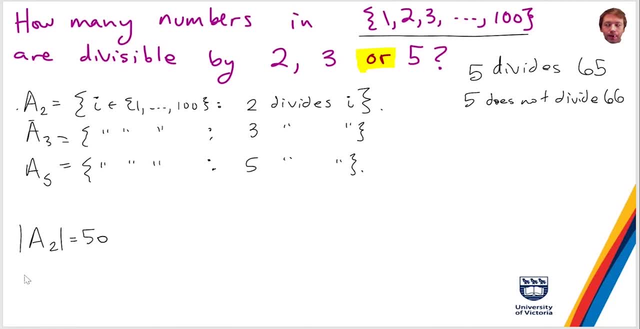 between 1 and 100 inclusive. So yeah, so it's 50.. How many are divisible by 3?? This one might take a bit more thinking. Yeah, 33,, because it's all the numbers you know. 3,. 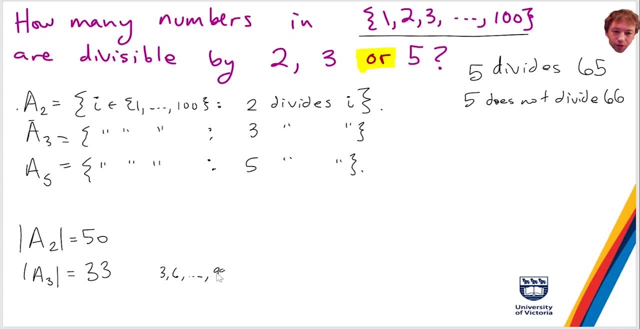 6, blah, blah, blah up to 99. So it's like 1 times 3, 2 times 3, up to 33 times 3 are all between 1 and 100.. So that's 33 numbers. 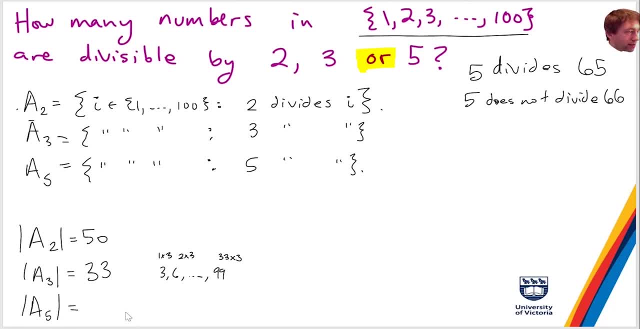 A5, right, it's going to be 20, right, Because I got 1 times 5 all the way up to 100, which is 20 times 5.. Okay, what about A2 intersect A3? Probably 16.. 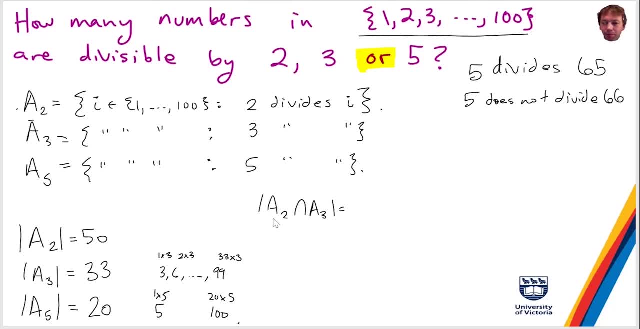 That looks right. right, Because if a number is divisible by 2 and by 3, that's the same as saying it's divisible by 6, right? So we've got 6, which is 1 times 6.. We've got 2 times 6,. 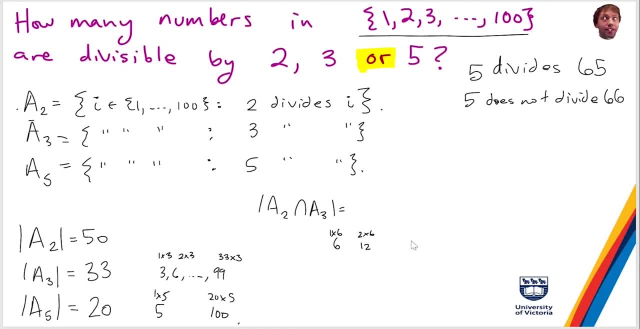 which is 12,, all the way up to what is 16 times 6? 96,, I guess something like that. So we've got 16 times 6, which is 96.. So yeah, so this is 16.. 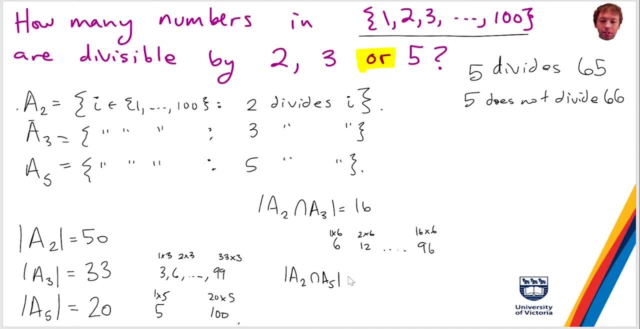 Similarly, A2 intersect A5 is the is the multiples of 10.. So there's 10 of them. A3 intersect A5 is the multiples of 15, 1,, 2,, probably, probably, 6 of them. 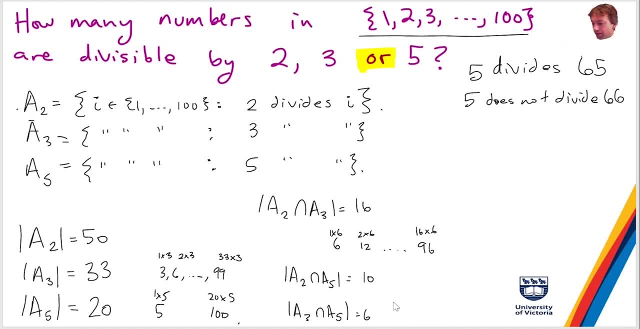 right, Everything from 15,, 30,, 45,, 60,, 75,, 90,, that's 6.. And then, how big is A2 intersect, A5, intersect or, sorry, the intersection of all of them, A2,. 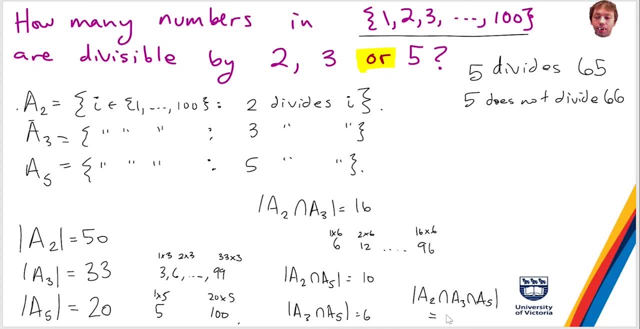 A3, A5.. So that's the multiples of 30. So that's 3.. Okay, putting it all together, we use inclusion exclusion to say that the answer is 50 plus 33 plus 20 minus. where did I write all this stuff? 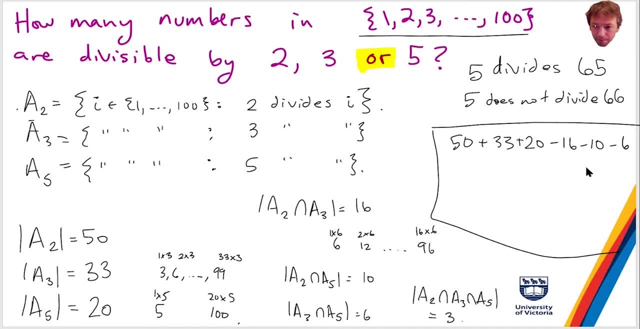 16 minus 10 minus 6 plus 3,, which is something I have no idea. but okay, So is it clear. Yeah, I'm not going to compute the number because, okay, I'm just going to get it wrong and confuse people. 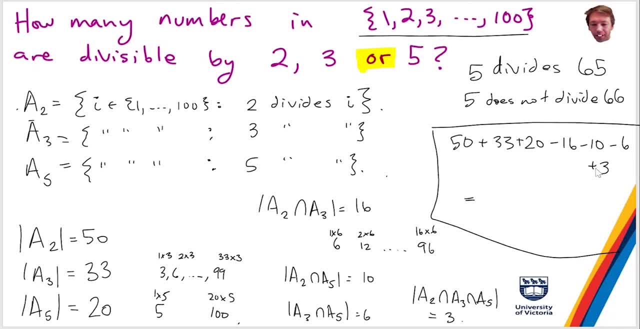 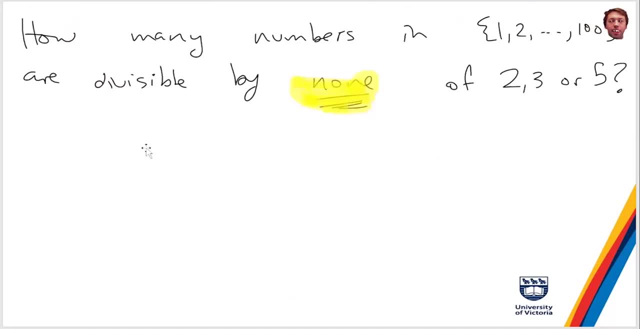 but but yeah, this you can put into the calculator and you're going to get the right answer. Okay, Okay, Okay, Yeah. How many of the numbers in 1 to 100 are divisible by none of 2,, 3,? 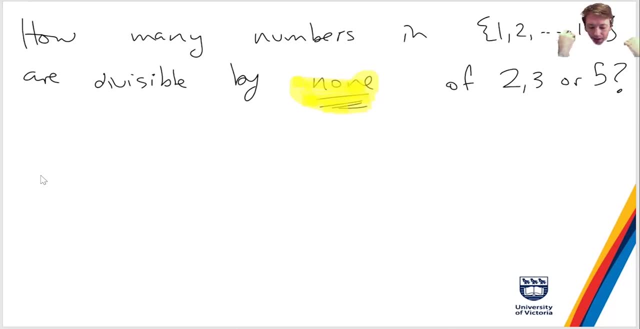 or 5?? So that's like I'm trying to illustrate something here. that right. So inclusion, exclusion, tells you how to like, compute the things which are like, count things which are like one thing or the other, or the other or the other. 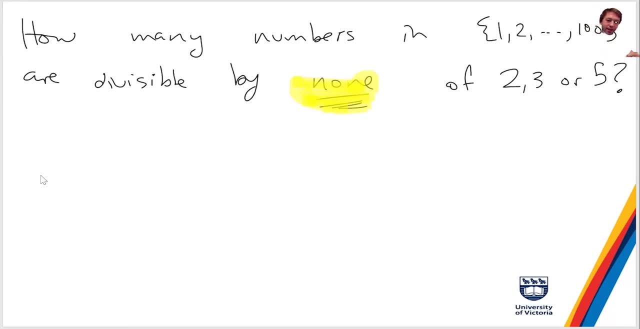 but you can also count things which are neither the first thing nor the second thing, nor the third right, Or and so on, because- and the way to do this is just to use this standard kind of rule of well- 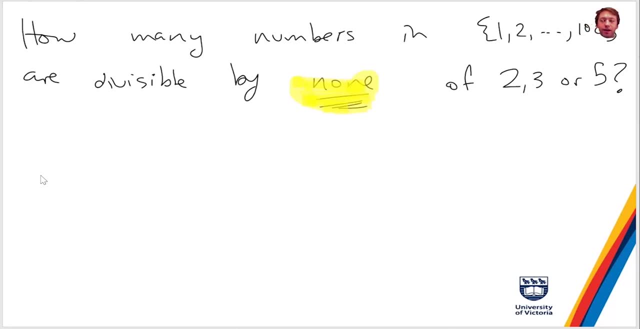 counting the compliment. So what you want to do is take the total and subtract the ones you don't want to count. So here my total is a hundred, right, And I want to avoid counting the things which are divisible by 2,. 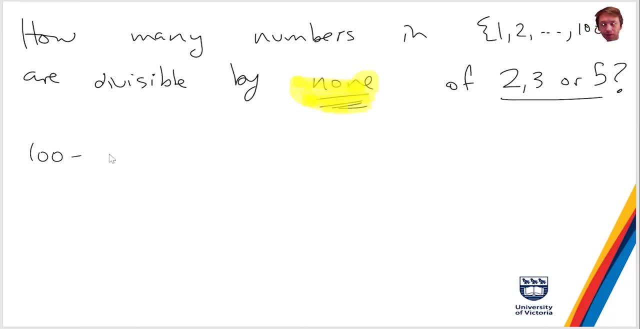 3, and 5.. So I just have to subtract them. So so it's minus, like whatever. this was 50 minus 33.. So, or maybe I'll- I'll write it like that: So minus with a big like bracket, 50 plus 33,. 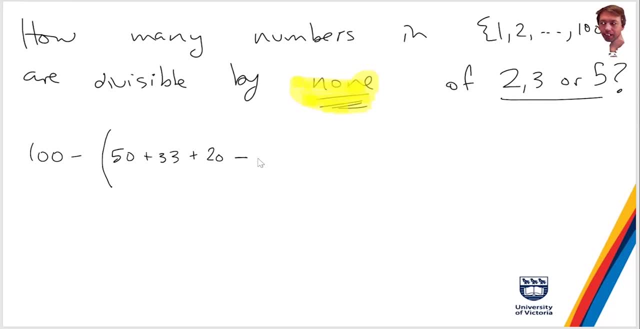 like so. now I'm just doing the same thing We just did, counting the multiples of 2, 3, or 5 minus 16, minus 10, minus 6 plus 3.. And then again this is equal to something. 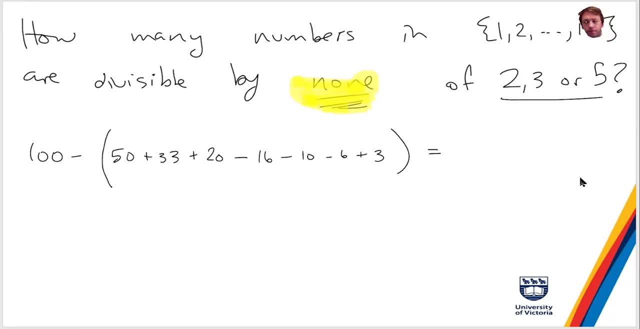 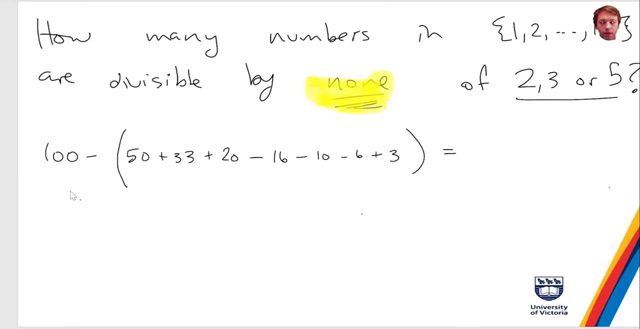 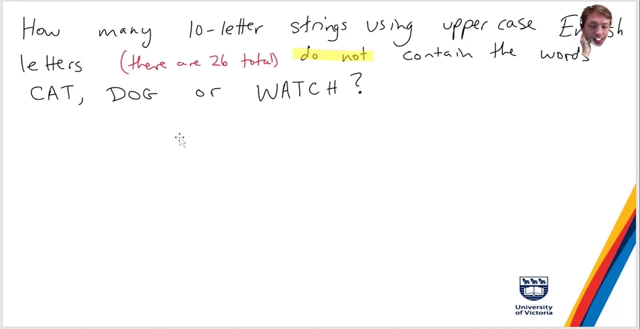 but yeah, is that clear? Okay, So, okay. So I've got just a few more examples to to deal with. So, yeah, So how many 10 letter strings using uppercase English letters? So remember there in English we have 26 different letters. 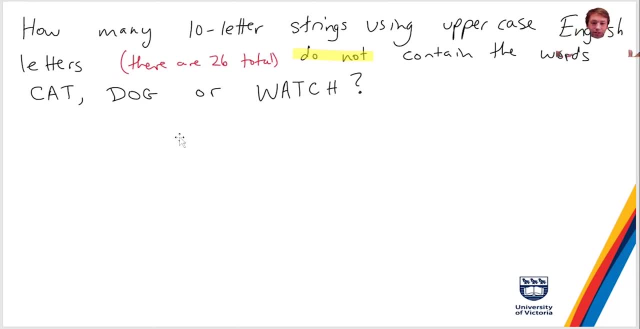 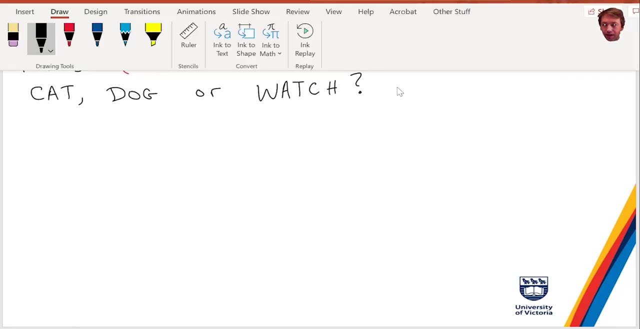 And we're only using uppercase, So there's only 26 choices for each letter, And we want words that do not contain cat or dog or watch Right, So meaning yeah the like if I. I wrote Zed. 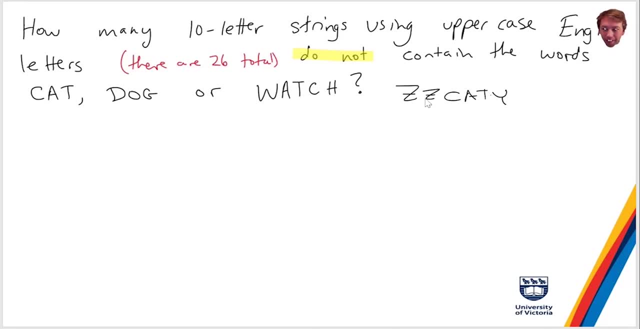 Zed cat Y. so 1,, 2,, 3,, 4,, 5, Y, Y, Y Y, like this is forbidden. An example of a forbidden word: right. Or if I wrote, cat. 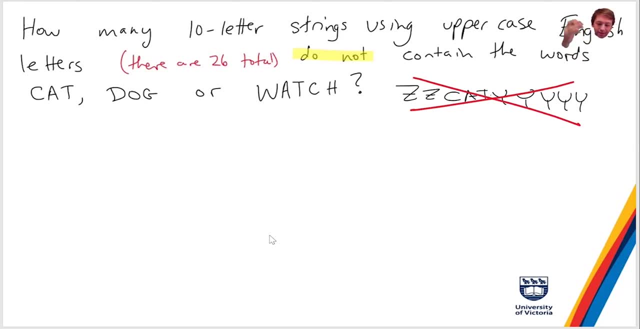 or like watch cat and then X, B or something, then that's also forbidden. Okay, So how many words are there that forbid all of these sub words? or they forbid all of these strings? Well, again, we want to count the compliment. 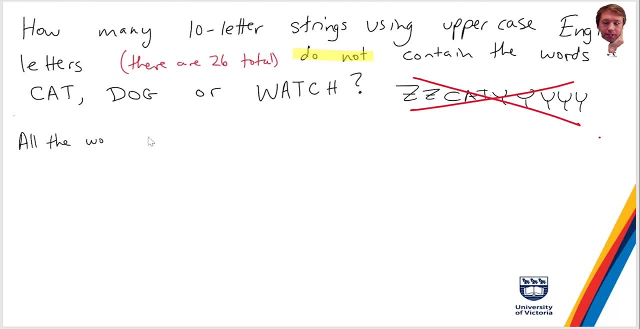 right. So we want to take all the words or all the strings, or whatever, with no, with no restrictions, So with no restrictions. So how much is? how many are there? So, as usual, we have 26 to the 10.. 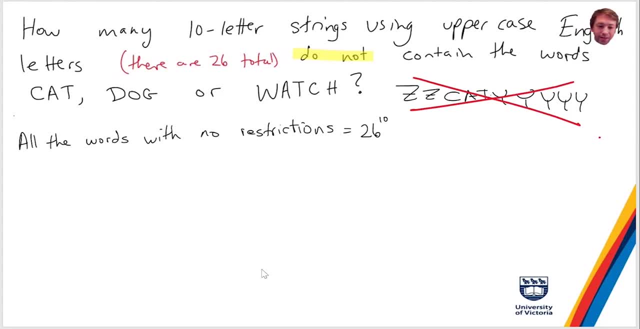 So we have to keep remembering this is not 10 to the 26. It's 26 to the 10.. Okay, And we want to subtract the bad words, like the words that contain the forbidden sub words. So how many contain C, A, T? 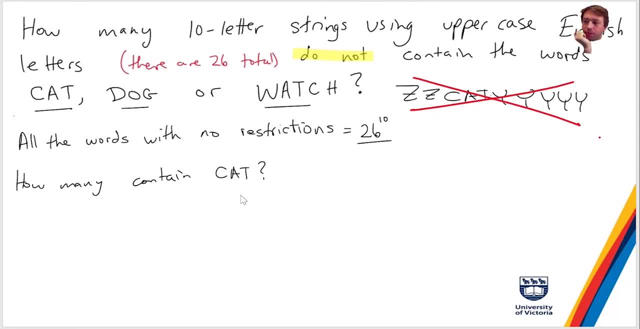 Any ideas? Maybe not trivial, takes a little bit of thinking. but how many 10 letter strings contain the word cat? So, and when I say it contains, like they have to be consecutive letters, like it has to have a C, A, T. 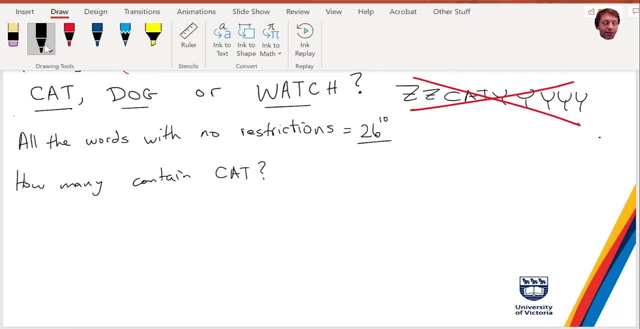 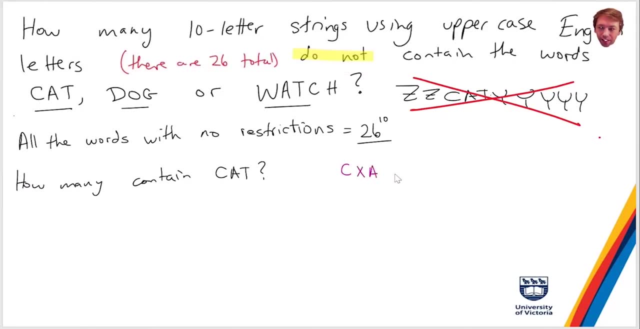 So yeah, this would be the. so there's an answer in the chat, which would be the case if I. so I don't want to, but I don't want to count things like C, X, A, R, you know, T, like where it's that letters are separated, and then whatever else. 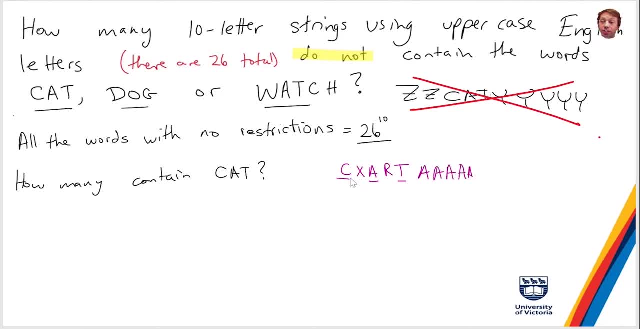 like A, A, A right Cause. if you're doing eight, choose three. you'd be choosing. potentially you would be putting the letters of cat in positions which are not consecutive. Yeah, So probably if I, if I was giving you this on an assignment. 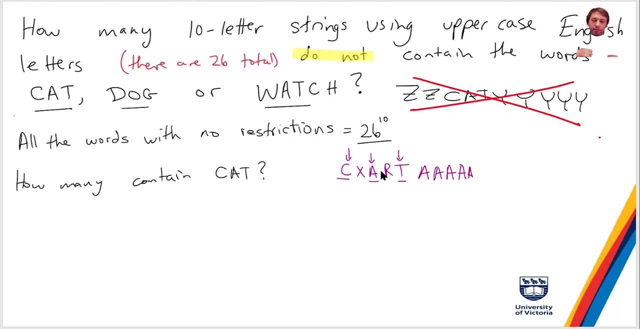 I should make it more clear what I mean by containing the words. But when I say containing the words, I mean where the letters are consecutive. Okay, So so the eight choose three is so eight choose three. 26 to the seven is not quite right. 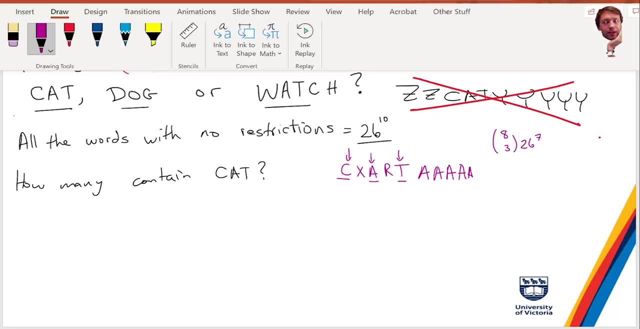 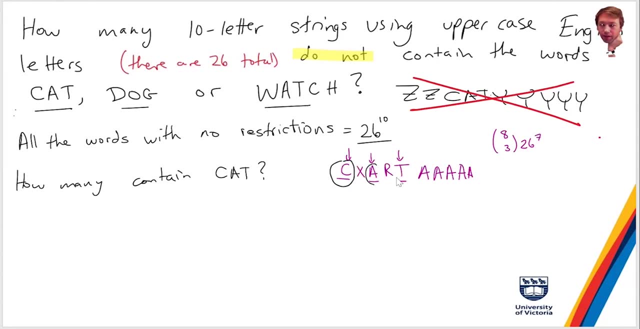 Eight choose three is not going to, because if you think about it, how many ways can I choose the position of cat? So if I was, if I was doing it like this, like if I had non-consecutive letters, this would be eight choose three. 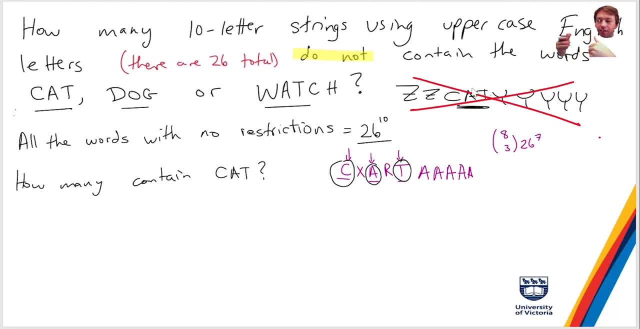 but I'm. the things I'm forbidding are where the letters come together. So, actually, if I the number of ways to choose where to put the cat, the word cat- is the number of ways to choose the first letter, which is actually just. 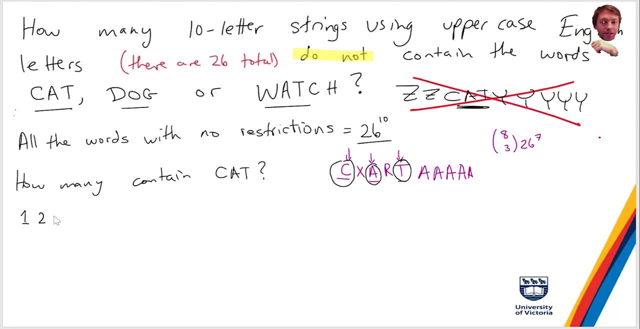 so the first letter could be, you know, start. it could start at the first letter, or the second, or the, you know. the C could be one, two, three, up to the eighth character, right? So actually there's only eight. 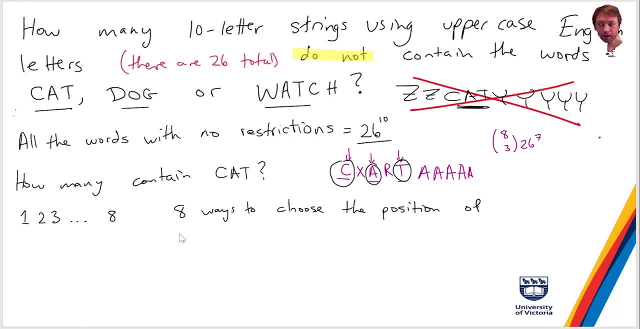 eight ways to choose the position of the word cat, If that makes sense, because the C can either start on the first letter, second, up to the eighth eight, choose three would not be the right thing because it's it's choosing. 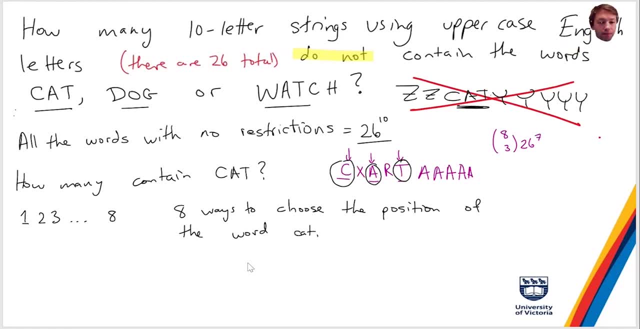 you know, it doesn't necessarily put them consecutively. So I'm actually realizing that this problem might be might be harder than I anticipated, but let's, let's go through it anyway. So right, So you get well. 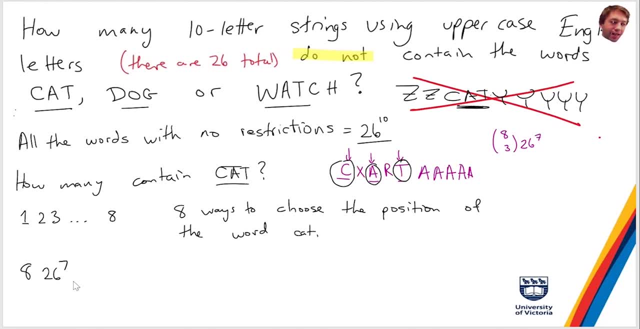 if I do write eight times 26 to the seven, that looks right, but it's actually not quite right, Because if you think about it, how many times did I count this word Cat, cat, B, B B. 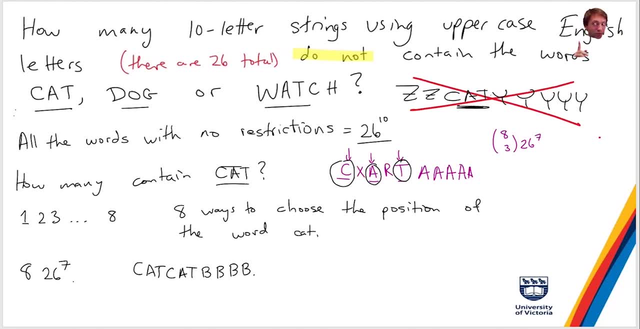 B And if you think about it, I actually I didn't just count this once, I actually counted it twice, because I I counted it once by saying, okay, I'm going to say the cat is here And then I choose whatever I want on the rest, 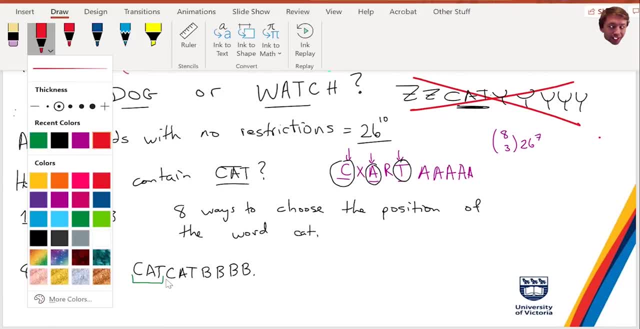 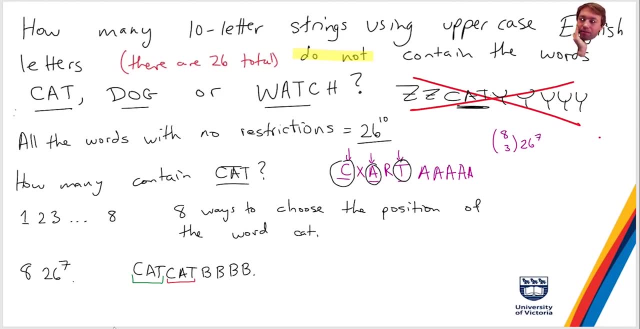 And I chose, and I also counted it by saying: okay, put the cat here and do whatever you want on the rest, Okay, So you have to be very careful with these things, because- yeah, because this would count these things the wrong number of times. 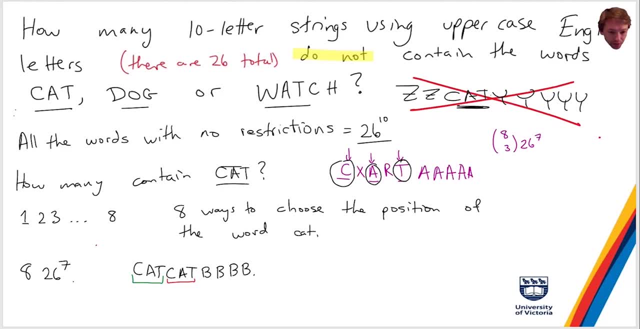 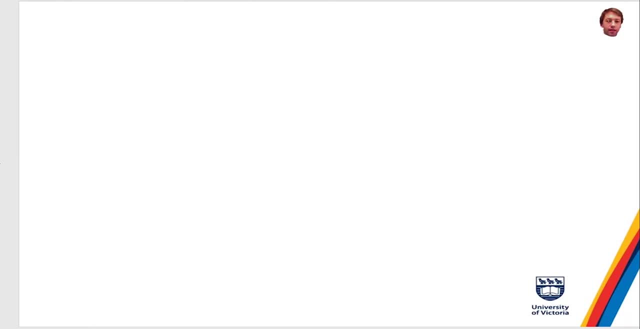 right, It'll count it twice, Okay, So what I'm going to do? um, okay, let's come back to that If we have time. probably, we probably won't, Yeah. So actually this, this question is a little bit tricky. 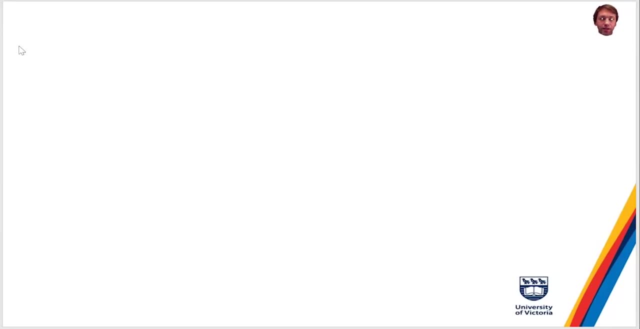 So what I'm going to do is to count the number of words, that the number of words that have the number of strings that have cat in it. What I'm going to do is I'm going to say, let A I be the number of. 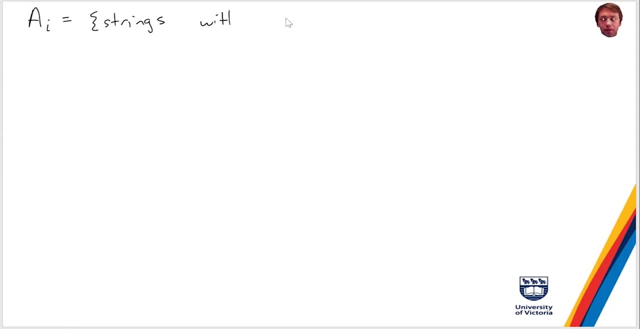 be the collection of all strings with the word cat. Cat starting at position I. Okay, So this is for I, between one and eight, because cat can't start at the ninth position. right, Because it's not. you know, it's too long. 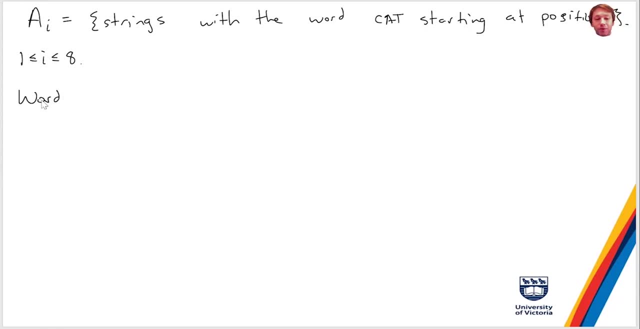 So actually the the words, so the strings, with cat in it is going to be the union. I equals one to eight of A I Okay. So this is actually kind of you kind of have to do this If you're going to want to count this correctly. 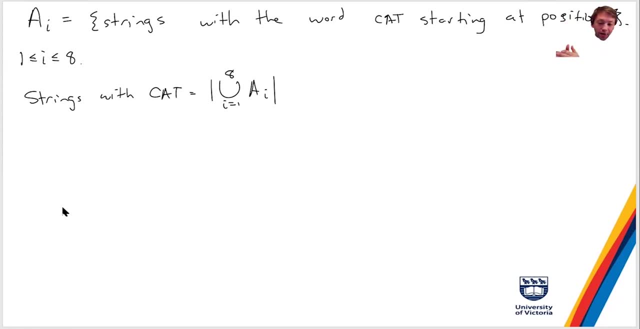 because, like I said on the previous slide, if the word cat appears twice, if you, just you know the, the original thing we had, which was eight times 26 to the seven, that's going to count those things, the wrong number of times. 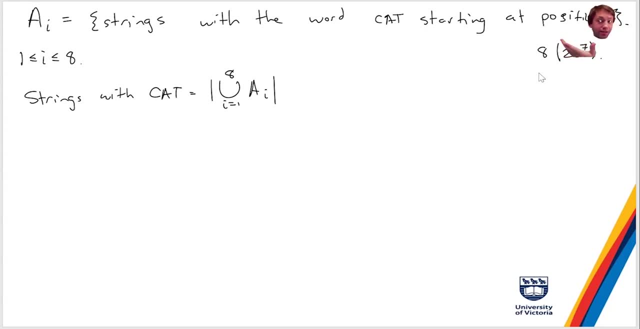 It's going to count it twice, And if it has the word cat, three times it's going to. that's going to be a problem as well. So so right. So this is equal to um. well, how big is? 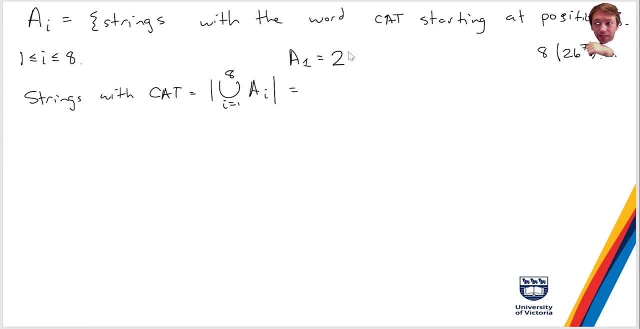 let's say a one. Well, that one actually does have. so the size of that is 26 to the seven, because I just put a cat on the first three letters and I choose the other ones And in fact all the AIs have the same size, if you think about it. 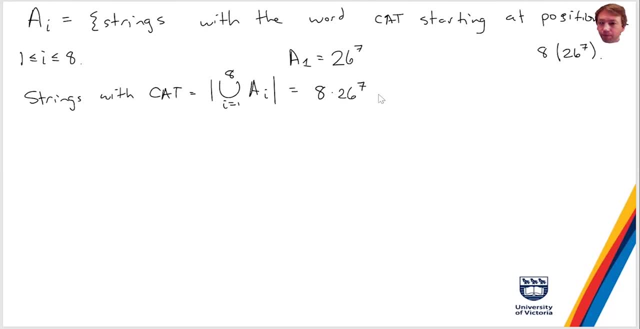 So this is eight times 26 to the seven. but then you have to subtract the intersections. So how big is? here's a question: How big is A1 intersect A2? So you guys with me here, How many words have the word cat, starting on the first character and on the second? 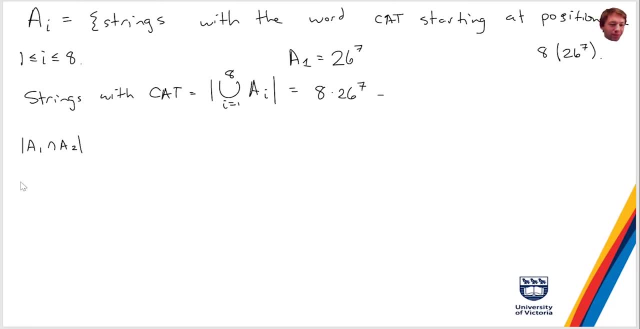 It is slightly a trick question. Yeah, the answer is zero, because if it's, if it starts with CAT, well that's not a C, So I can't have CAT. you know here as well. So so actually, 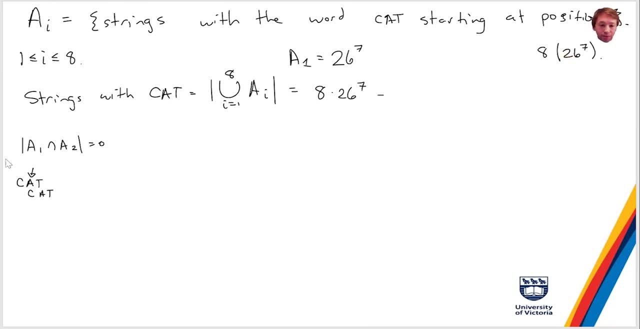 yes, this is zero. In the same way, A1 intersect A3 is zero. What is A1 intersect A4?? So I think it's not zero, because I could go cat, cat and then I've got yeah. 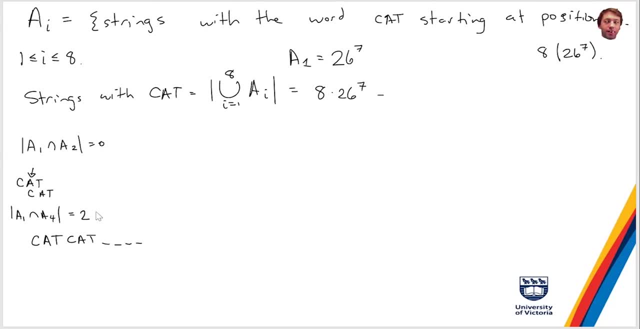 I've got four characters left And so yeah, then I'm good. So so I got 26 to the four and the same. if, if I take A1, intersect A5 or six or seven or eight, and then 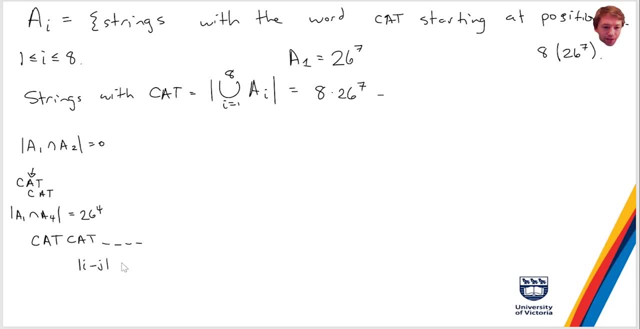 so basically, if I minus J is at least three, you get like A. I intersect A. J is 26 to the four. And oh dear, how do I count that? But anyway, it's going to be 26 to the four times something. 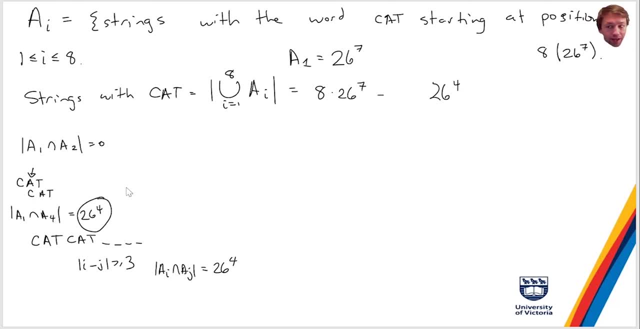 Well, how many? so I've got four, five, six, seven, eight. So I've got five things that like if, if if I'm dealing with A1 intersect something, there's five good sets, Like there's five. 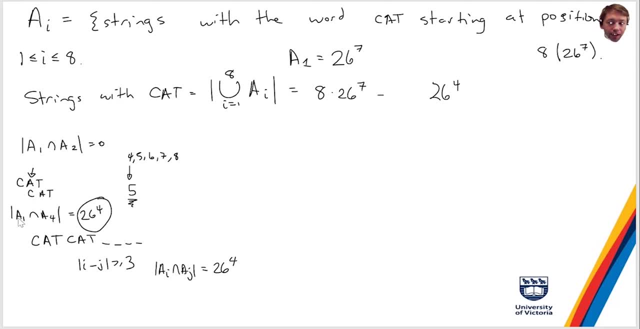 like you know, four, five, six, seven, eight, like A1 intersect. any of these is okay, If you think about it. A2 intersect. anything is okay, As long as it's not so. four is not okay. 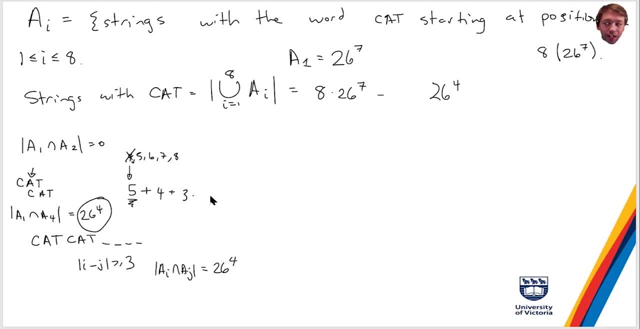 but anything, five, six, seven or eight is okay. Anyway, you get the coefficient here You're going to get is like this: So it'll be six times. So remember, we, we, we computed the sum of one up to N. 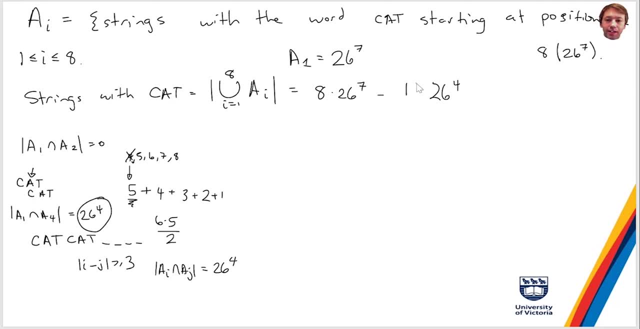 right, It's N plus one times N over two, So that's actually going to be 15.. So sorry if you don't catch all these details. I'm just going a bit fast because we're practically out of time, So I think I won't be able to finish this one. 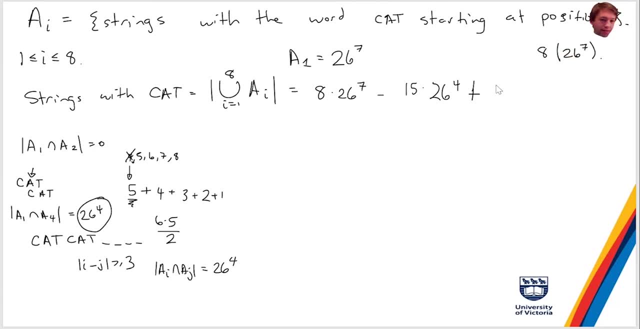 But if you have three counts, well, that's going to fill up the entire string essentially, except for one character. So basically, you just choose the character too. So I've got 10 choices for which character is not part of the cats. 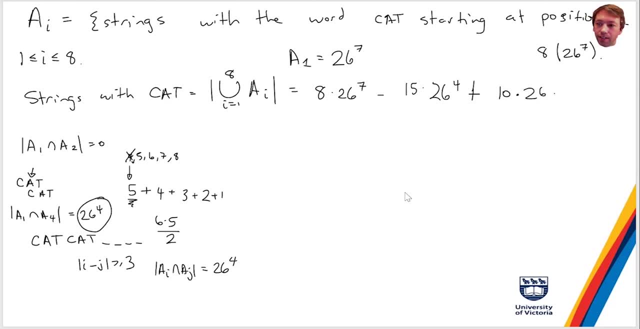 And I take 26 and okay. So this counts the strings that have cat, Okay, Which was already pretty complicated, And the strings that have dog is going to be the same. The strings that have watch is going to be a bit different.